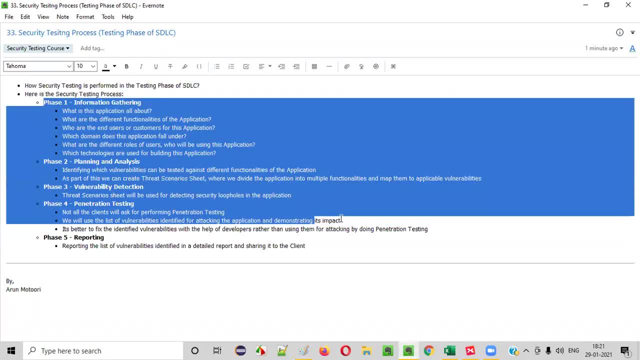 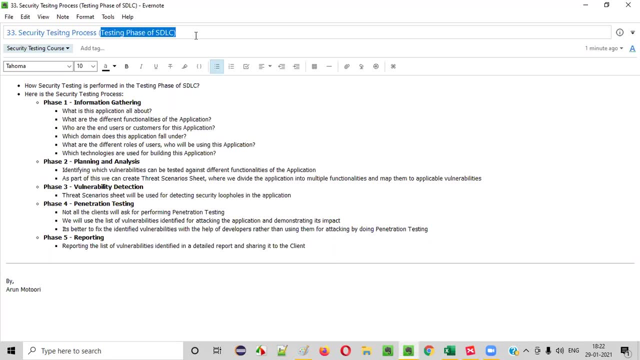 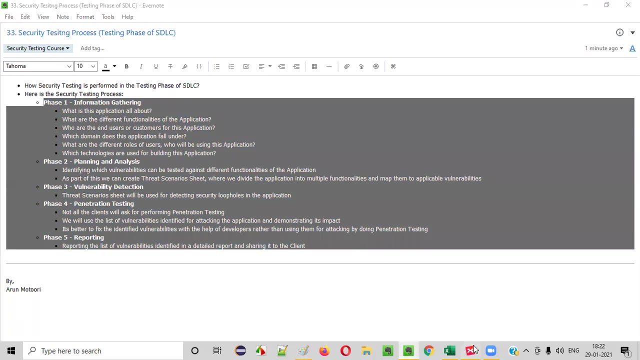 application is stable for security testing, then here is the process, guys, here are here. there are five phases. okay, we are going to perform security testing in this testing phase of sdlc, in this five phases, guys that are listed on here. let me show you a better view of this particular phases in. 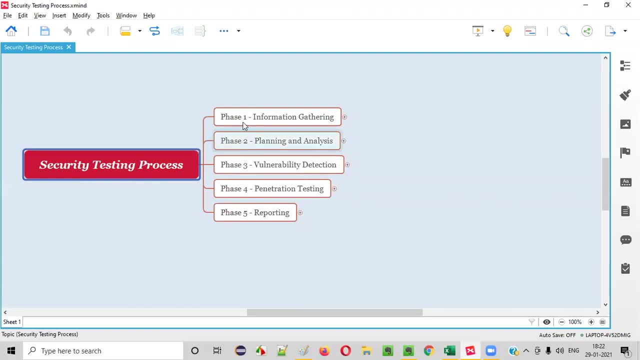 this mind map. as you can see, security testing process can be categorized into five phases. okay, we'll see you in a minute. start with the phase one. after phase one is done, we'll go to the phase two. after phase two, we'll go to the phase three, phase four, phase five: okay, so to begin with, this is the first phase, guys. phase. 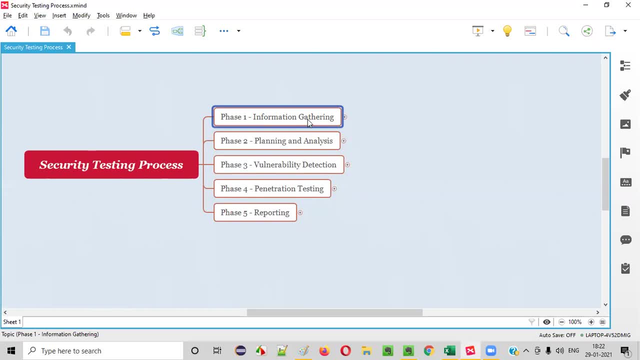 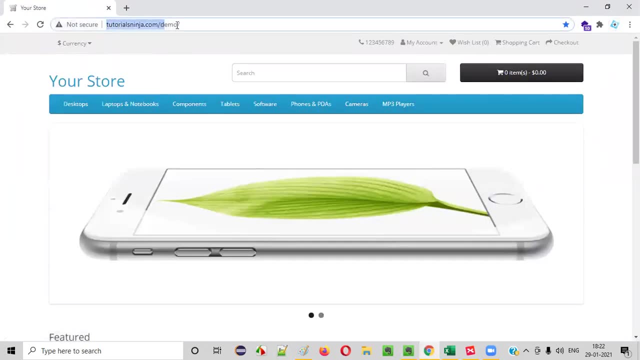 one is about information gathering. once you get an application as part of security testing, let's say: you got this application, guys. okay, let's take this as an example. okay, let's take this particular application as an example. tutorials in your dot com slash demo when you get this. 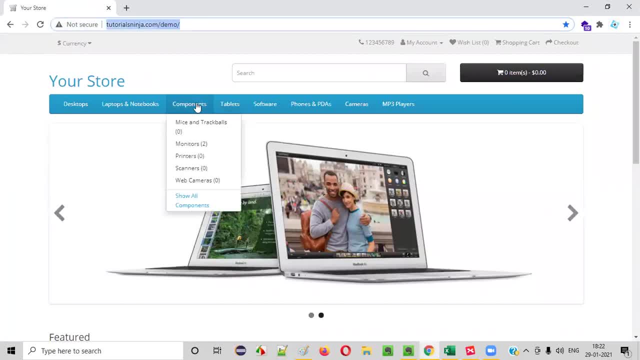 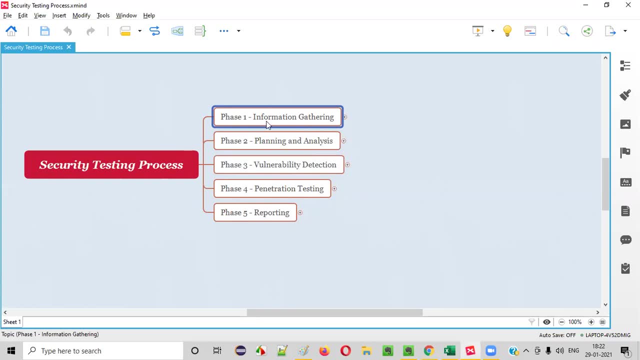 particular application as part of security testing requirement, then the first thing that you would do is you'll first gather, okay, information, first you will gather the information. that is information gathering phase, guys. okay, the first phase of security testing process as part of real-time working in any projects. right, the first phase is going to be: 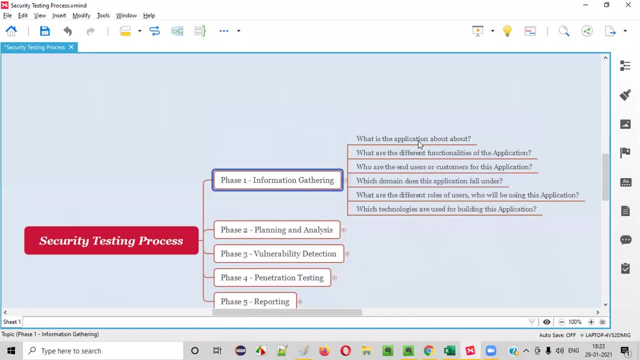 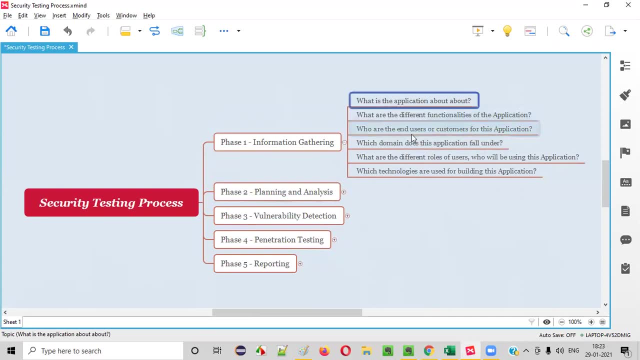 the information gathering phase where you are going to answer all this stuff. okay, in the first phase of security testing process, you have to do this information gathering where you need to answer all these questions. the first question is: what is the application all about? so let me, let me show. 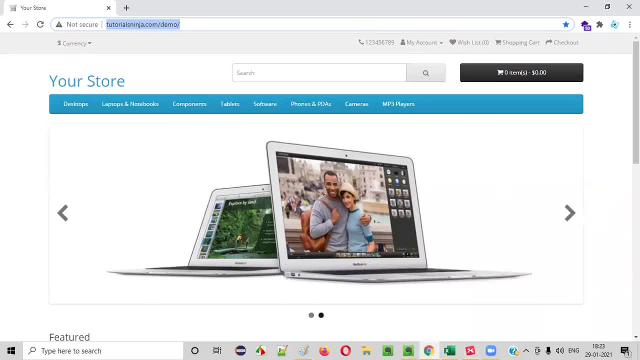 you this application and then we'll understand these questions and try to answer. okay, let's say, this is a demo application, example application, and you see what is the application all about. this application is all about selling the products online. okay, so this tutorials in your dot com. 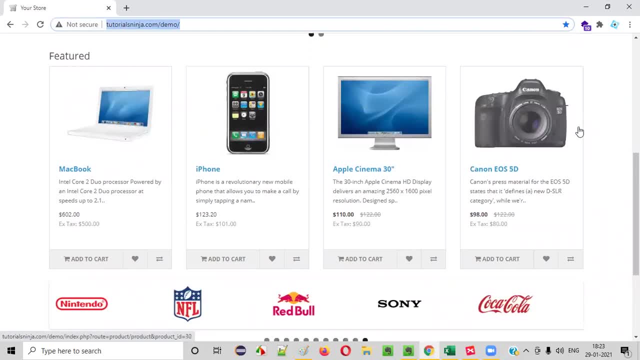 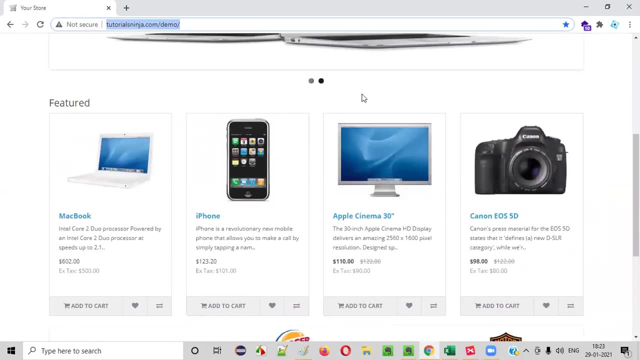 slash demo application is selling this particular products online guys. okay, so macbook, iphone, all these products are being sold. people or end users can purchase all these products from this website. this application is all about selling this product case. so we got some idea what. what is the? 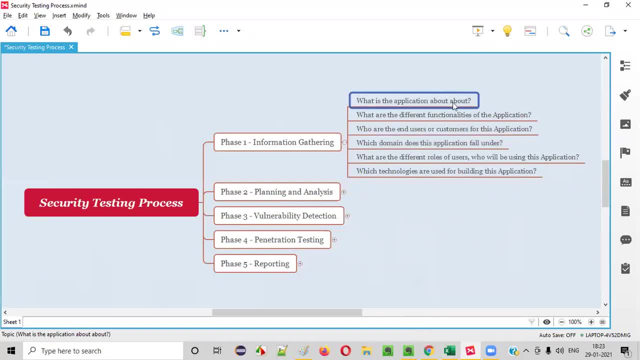 application all about. it's an e-commerce application where the products are different. digital products, okay, like digital devices, kind of products like iphone, mac laptops, desktops, cameras, all such kind of items are being sold on the website. so that is a purpose, okay. what is the application all about? you just understood? next thing, what you will note on. 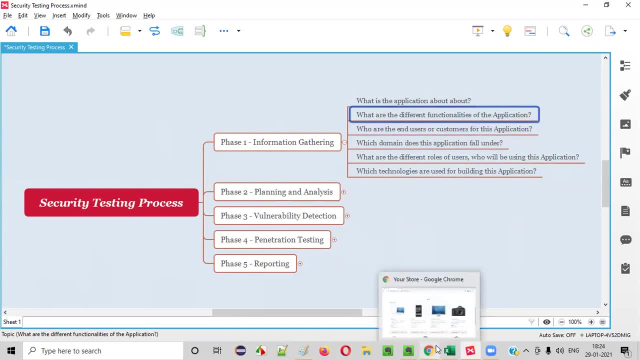 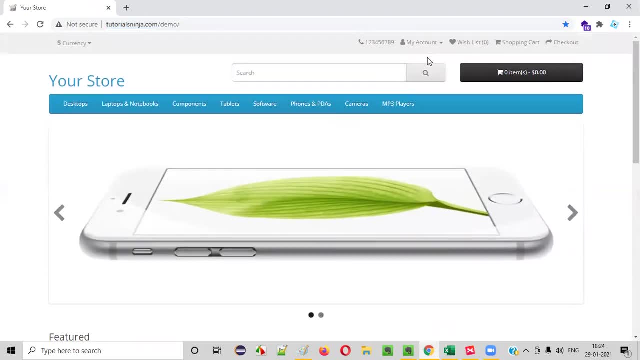 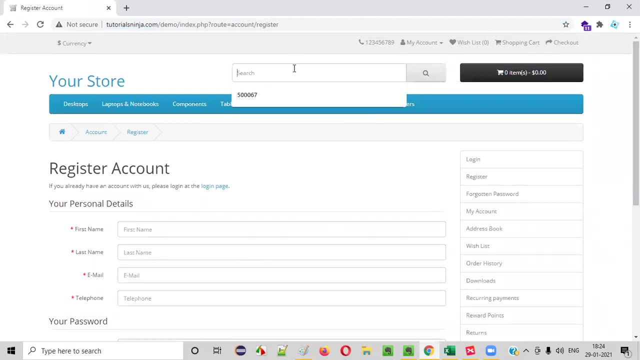 next thing is: what are the different functionalities of the application? so when you look at this particular application, this application has lots and lots of functionalities, guys. a few examples of the functionalities are like: this has a login functionality. this has a register. you can create an account here. i like that. each and every functionality count, guys. okay, your search. 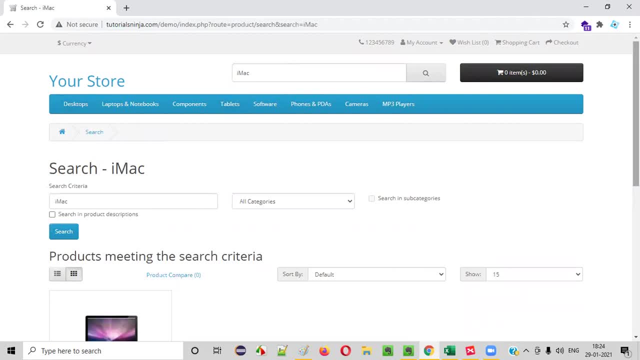 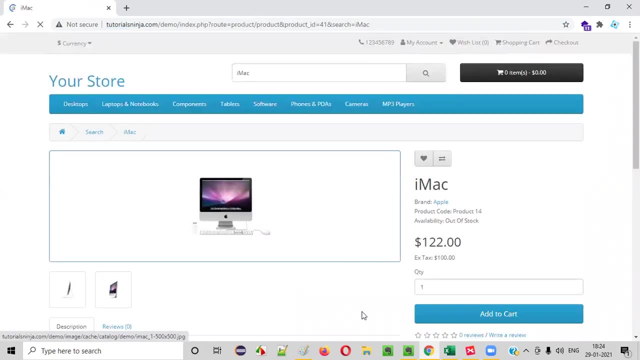 functionality is there. so we need to explore all this complete end-to-end functionalities of this application, like starting from the login, registration, searching, okay, then product display page functionality, and then we need to explore all these functionalities of this application. then adding this product to cart, shopping cart functionality- then we have shopping cart. 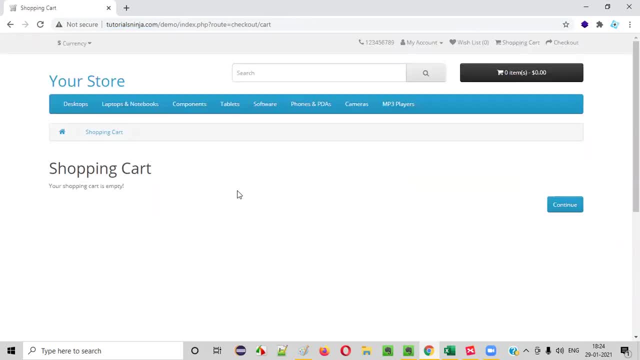 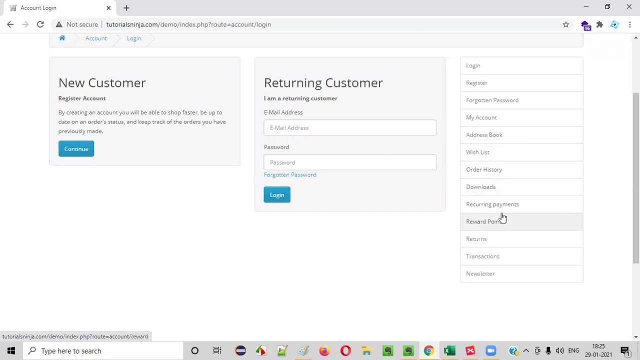 functionality and, uh, what else we have? okay, shopping cart functionality is there. uh, then checkout functionality is there. uh, then we, we can place the orders. a lot of stuff is wishlist is there? okay, which is functionality- is there? we can check the order history, downloads. uh, if you. 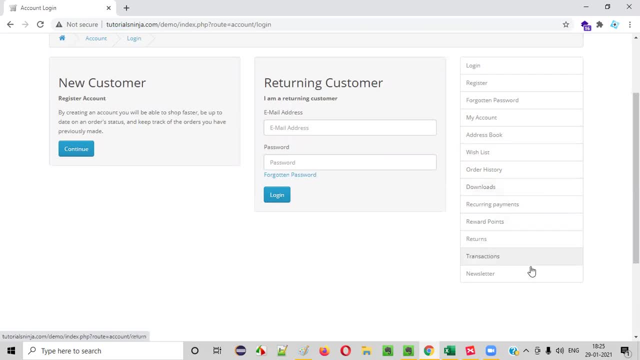 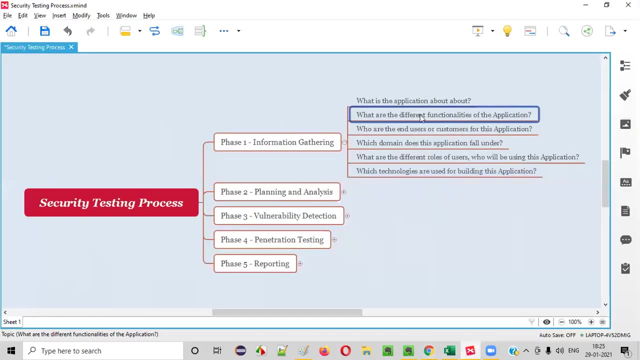 purchase some ebooks or some kind of things. they will be in the downloads guys. okay, so what is the recurring payment functionality? what is the reward points functionality, like that? a lot of functionalities are there. so we need to explore the application, guys, and identify all the different functionalities of the application. 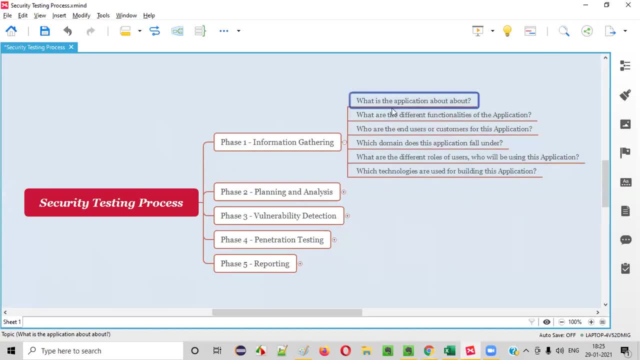 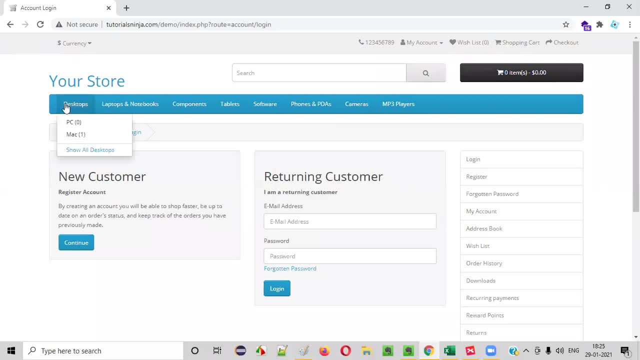 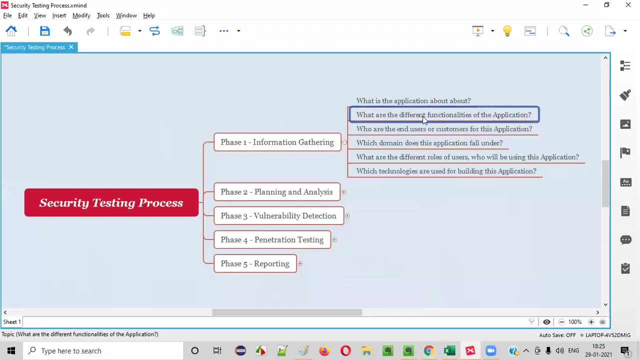 that is the second question. okay, so that means we need to spend enough time on this application, guys, as part of answering the second question, we need to spend good time on this complete application to see each and every functionality of this application. fine, fine, this is done, guys. 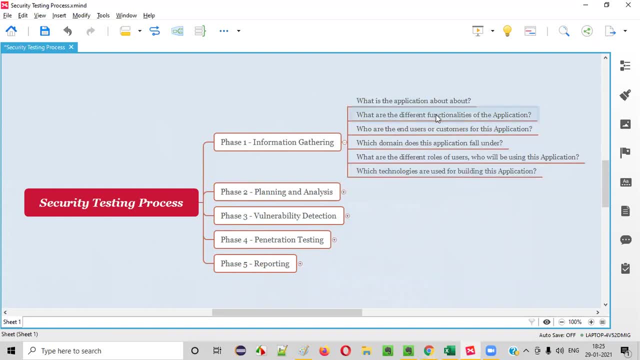 okay. so, uh, i'm just covering at a high level guys, uh, the live project, uh, the live project, uh live project thing where we'll be actually performing the secure testing will be coming in the upcoming sessions. till then, i'll just explain the concepts, guys. okay, once we start uh testing a real 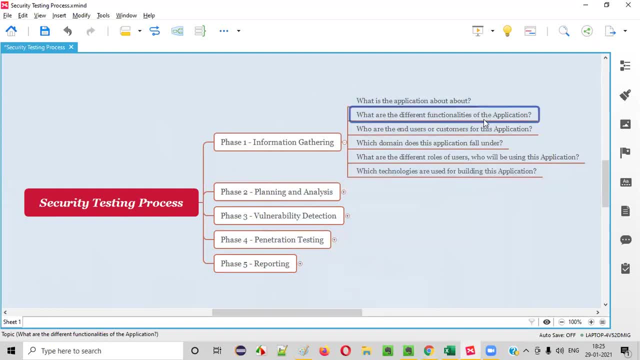 application, right, uh, then we'll go into the details, like identifying the different functionalities. okay, we'll go into the real time phase. okay, live project kind of stuff. but now just understand what, uh what we need to answer, okay, when you get an application for security testing. first thing, 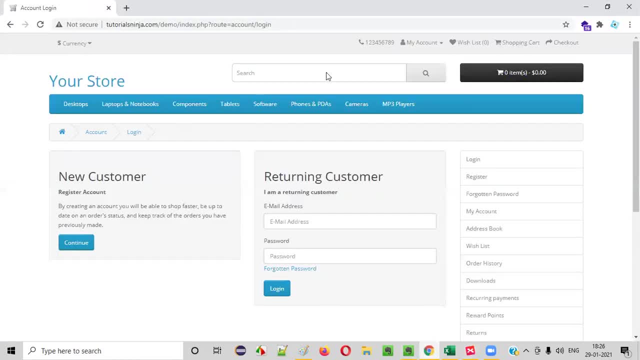 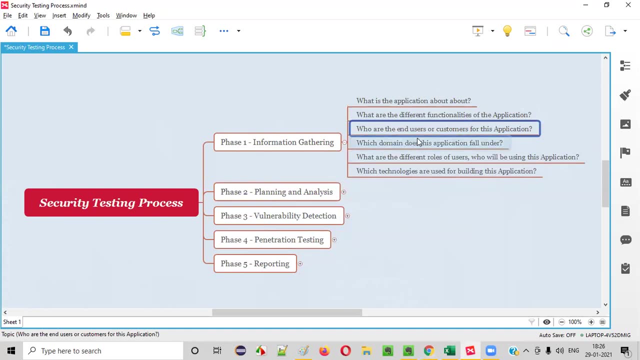 we need to know what the application is all about. second thing is: we need to identify each and every functionalities of this application at a high level. we'll go through okay. so third thing is: who are the end users or customers of this application? who are the end users, guys? the? 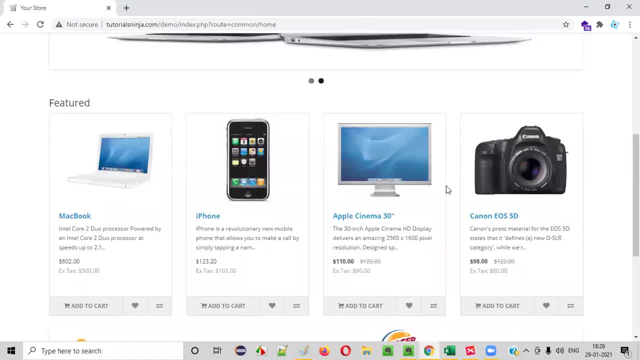 people who want to purchase these products are the end users. right, like that. we have to understand, okay, who are the end users, the customers who can purchase online. okay, any, any person who can purchase online is a end user. like that: we need to answer for different applications, different end. 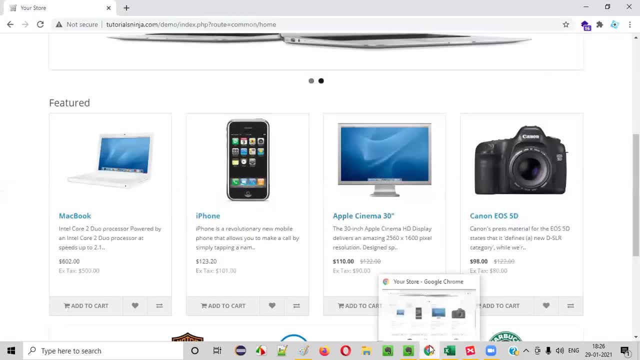 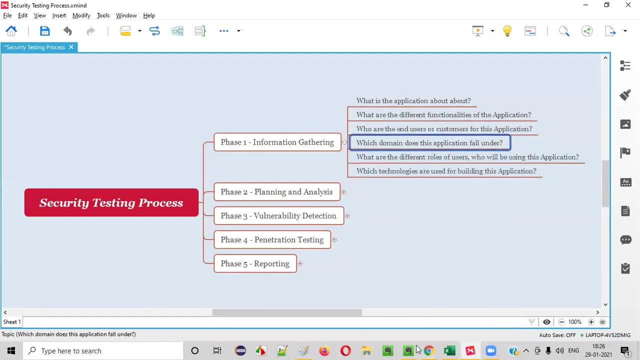 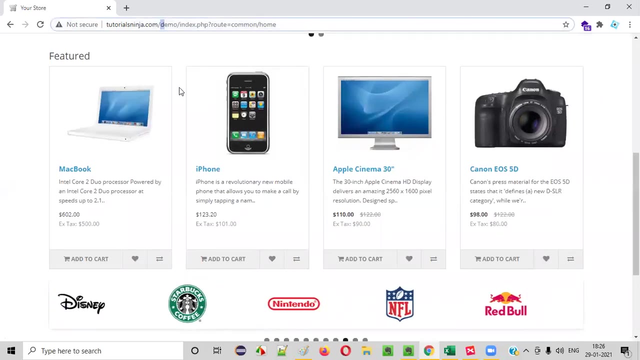 users will be there, guys, but for this e-commerce application, end users are the general customers who just purchase the things online. okay, which domain does this application fall under? this application that we are seeing here falls under the e-commerce domain, as we can see clearly see that this particular application is selling. 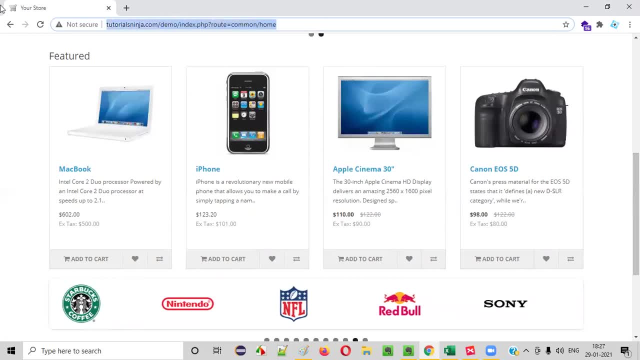 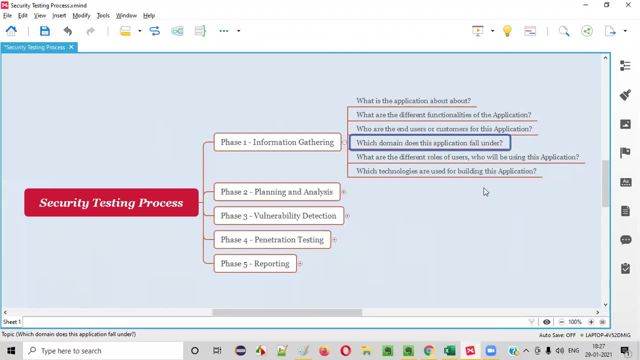 these products. okay, people can purchase these products online from this application. so this is an e-commerce application. so, similarly, there are different type of domains, uh, in terms of the applications like: uh, healthcare is there, banking is there? retail, is there a lot of domains, are there, guys? okay, this application falls under the e-commerce. 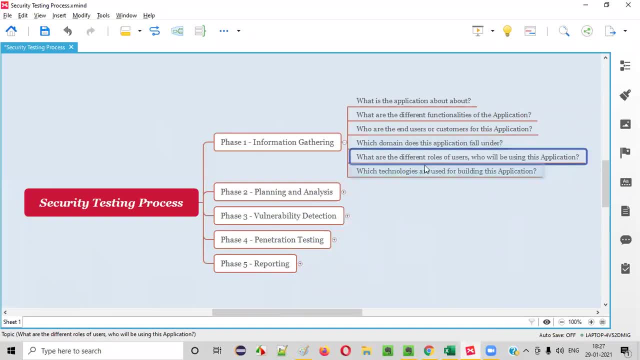 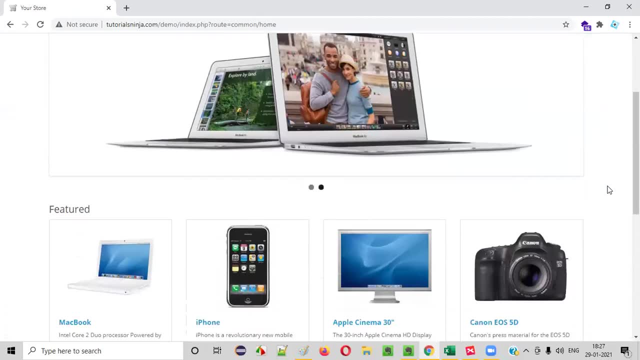 domain. and then what is the next question that we need to identify? what are the different roles of users who will be using this application? who will be using this application, guys? so if i ask you this particular question, you will be saying that end users will be using this application, right? 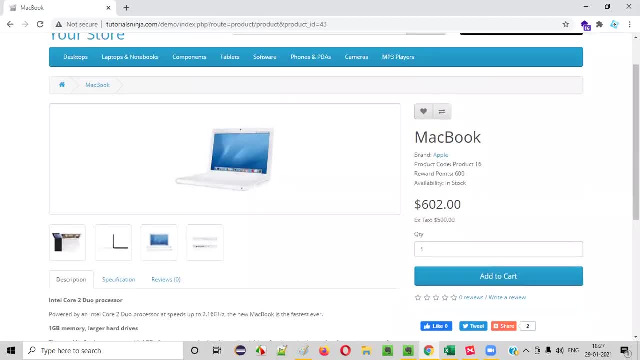 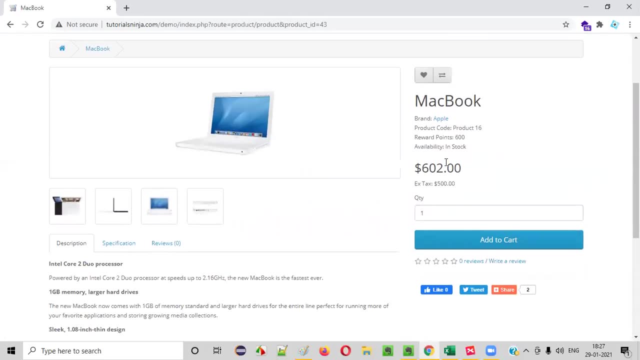 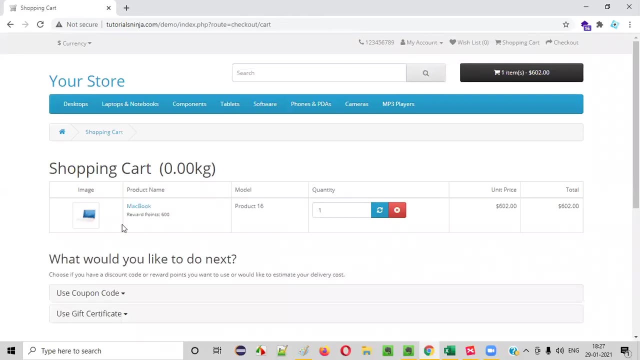 people like end users will be going to going through this application for purchasing the products. that is, one end user is a one user role and other users are also there, guys. for example, here, when you are trying to purchase this particular macbook or something you try to add to the cart, this item is there in the. this item is there in the inventory, guys. 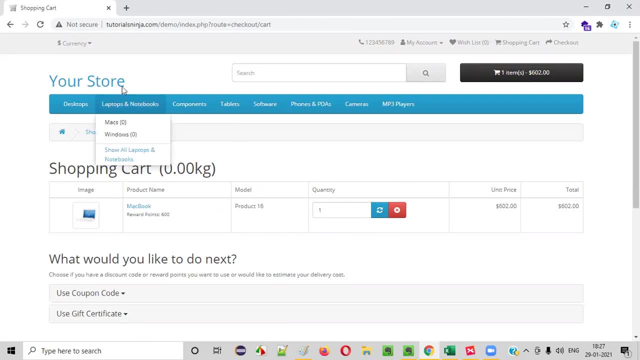 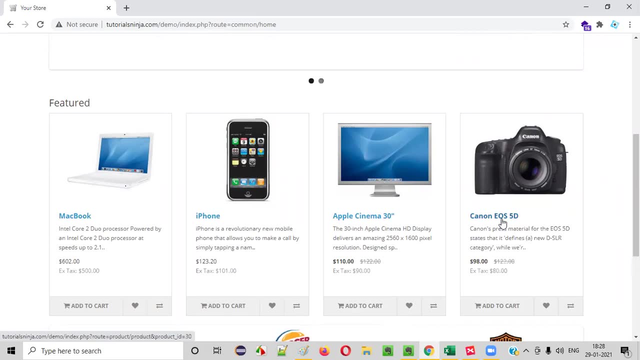 right, so few people need to add these items to this application tomorrow. in this list of items, guys, for now you are seeing this: macbook, iphone, apple cinema and canon right. tomorrow, if you see another product being added, who will be adding that product to this application? end user will. 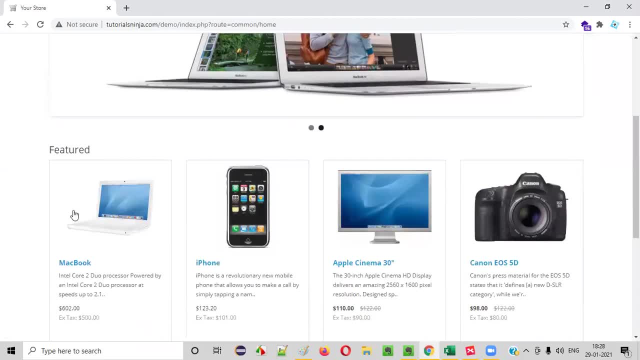 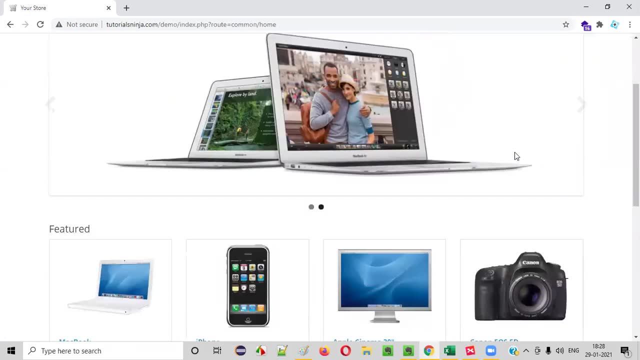 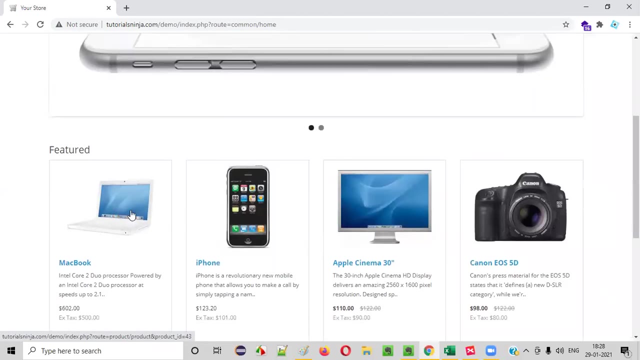 not be adding right. the people who are maintaining this application will be adding these products. okay, and kind of admin you can say- to this particular application. there will be some admin who can log in and add more products that can be sold from this website and also you can upload the images and he will write the descriptions. give the names of the. 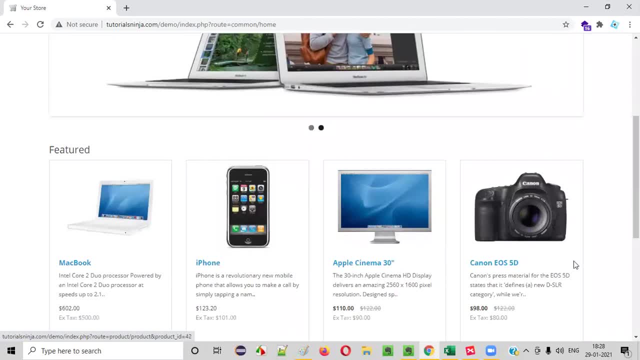 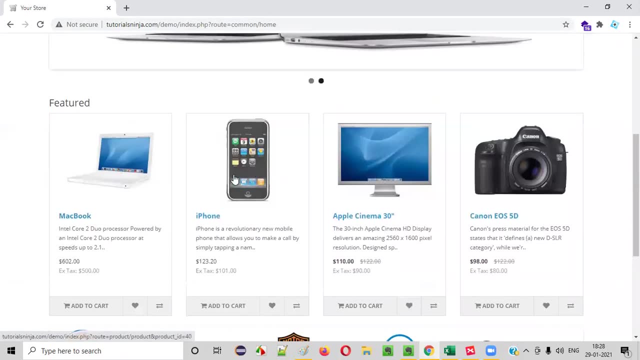 products, all those stuff. okay, maintaining the inventory and a lot of things are there. so here, two types of people i can see for this, particular tutorials in the application guys. one is like the end users, who generally purchase these products from this application, and another type of user. 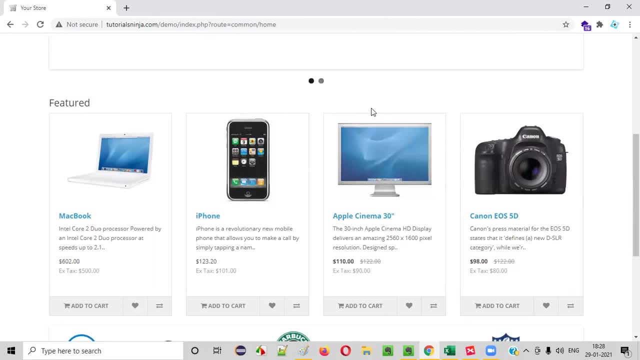 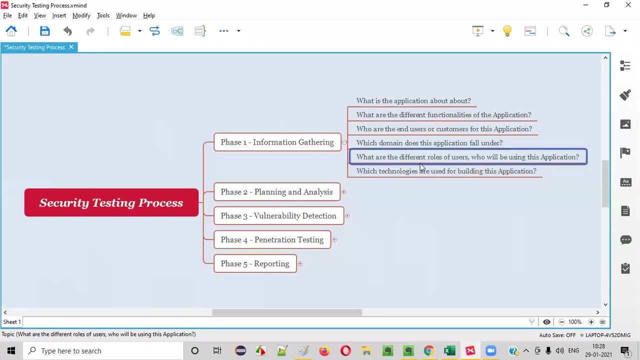 who will maintain these products in this particular application. he will add, update, delete the products. okay, all this stuff he will do on this particular application. so, like that, we need to identify who are the people who are going to use this application. okay, in our case there are. 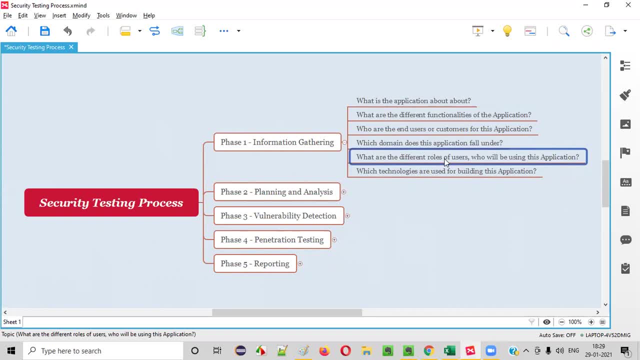 two rules in another case, for example, if you take some school website, who will be the user roles case? one user role will be teacher, one user role will be the student, another user role will be the admin, who will be adding the teachers and students. like that, guys, okay, it all depends on the real. 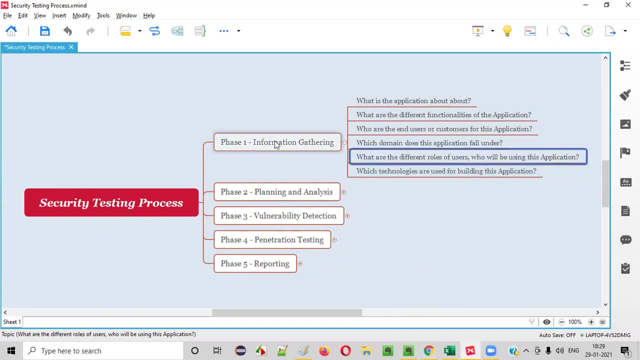 type of the application. so we, just as part of security testing process, guys, it's very important that we need to identify the user roles. okay, we need to get the details of the user roles who will be logging in and all the stuff, okay, so in the upcoming sessions, guys, i will explain like what: 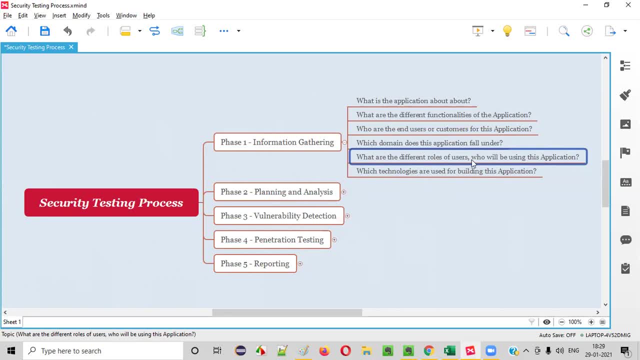 is the importance of the user roles and why we need to identify the user roles. okay, practically we will see. everything is from here to here, everything we are going to see practically. for now we are just covering at a high level in a theoretical way. okay, as much as possible, i am. 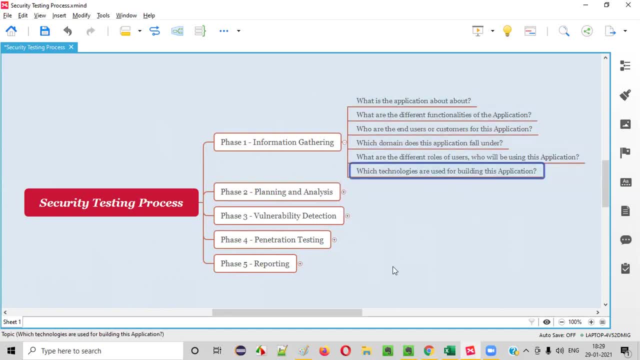 just going to demonstrate the stuff, but let's cover it at a high level. fine, so it's all part of the information gathering. guys, whatever i'm answering here is part of the information gathering. which technologies are used for building the application? okay, so as part of information gathering, apart from all this stuff, 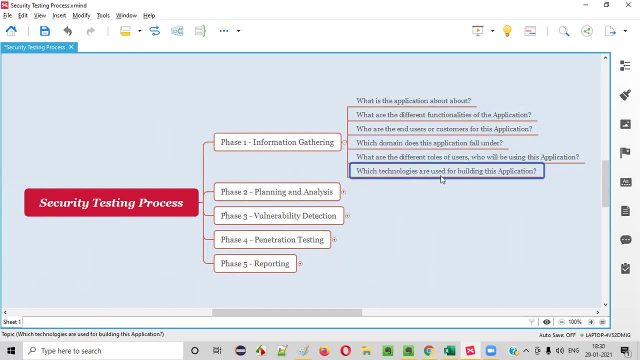 we should also gather the list of technologies, identify the list of technologies which are used for building the applications. okay, how to identify guys? how to identify the technologies which are used for building the application. let's say: this is application, right, so now let's say: you are at. 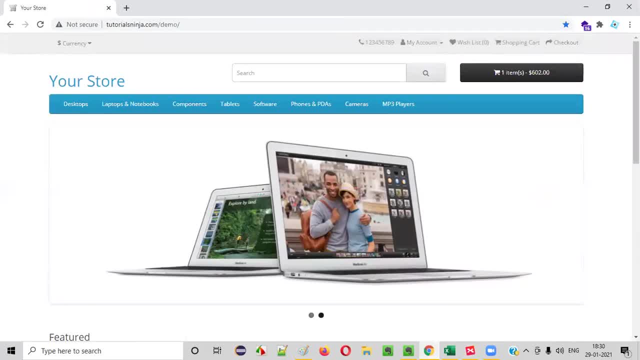 page. okay, now you want to just identify which technology is used for building this application. let's say: okay, how do you do, guys, by looking at this application, can you say which which technology is being used? by looking, sometimes you cannot say. so what we can do is we have to go to 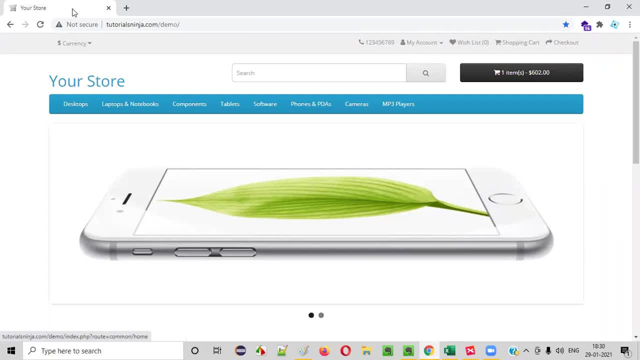 some different pages, guys, when you let's say, i'll click on this, your store logo of this particular page. so the moment i click right, this url got changed and in the url i can see some dot php right. so from the urls we can identify which technology this particular application is using. fine, dot ph. it's built using php and apart from 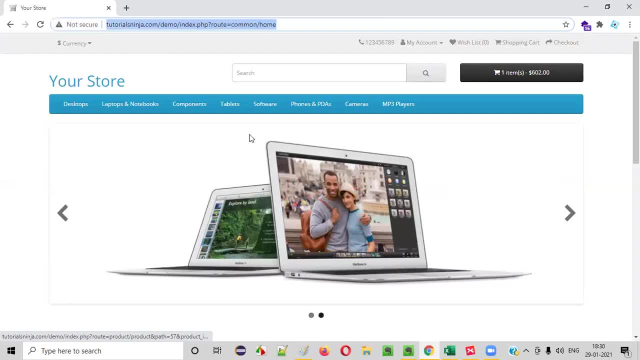 that, guys, if you are not able to identify using the urls, okay, because because of some security reasons, this kind of technologies may not be displayed in the urls sometimes. so in that cases you are not able to identify the which technology is being used for building this kind of application. 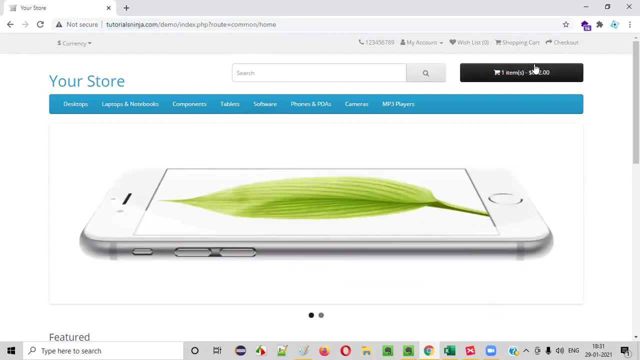 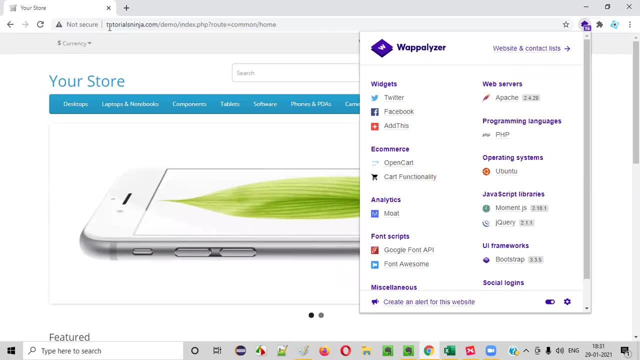 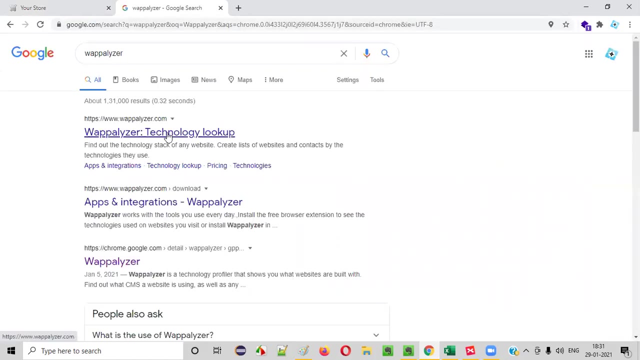 from the urls. then the next alternative is to install this kind of applications. okay, there's one application like uh vaporizer. okay, there's a chrome add-on. guys, you can vaporizer, vaporizer. so just uh, browse this. uh, you can go to the website directly, or directly, you can go to the chromegooglecom vaporizer. just click on that. 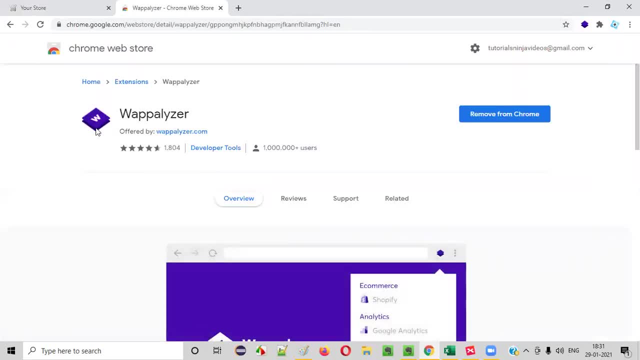 you'll be taken to the google chrome web store. you see, w is this kind of logo it has, and i already installed this. i already installed this add-on. this add-on will help you in finding all the different technologies that are used in your building your application. guys, i i will show you, like, how exactly the vaporizer is going to. 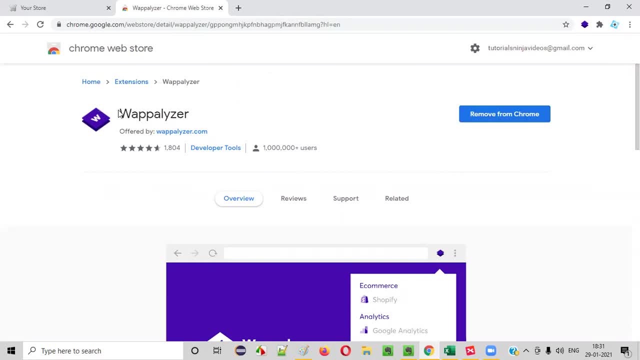 once you install, guys. i'm not going to show you how to install this, i already installed. just come to this google chrome web store and just install it- it will be there in your extensions- and just pin it so that you can directly see on the browser. that's it okay. so once you see on the browser, guys, 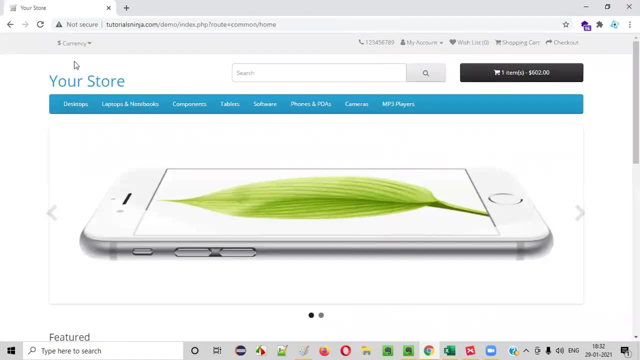 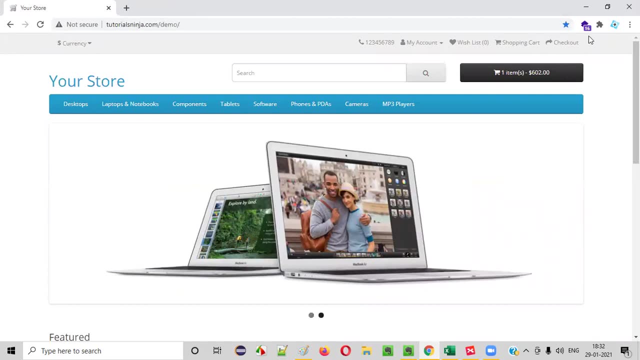 then, uh, simply refresh your browser and then, or relaunch your browser and go to the application like this: okay, go to the application like tutorialscom demo kind of application, and, uh, just click on this icon, guys. okay, click on this icon and then you can see that the application has been. 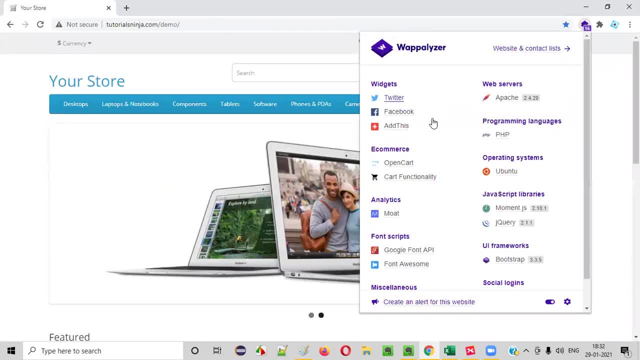 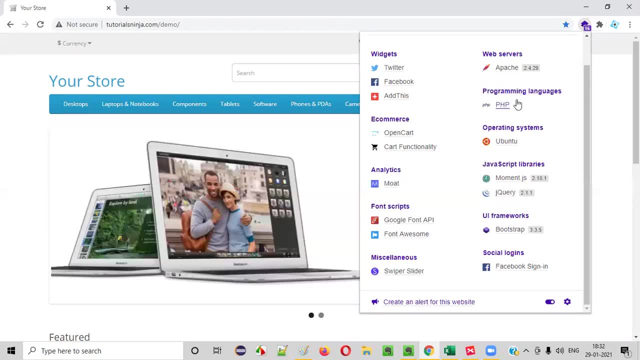 installed. okay, click on this vaporizer. you see all the list of items are listed here. okay, so it's giving you all the information about this application, like which programming language is used for building this application- php. you see it's directly. it will take some time, guys, okay. 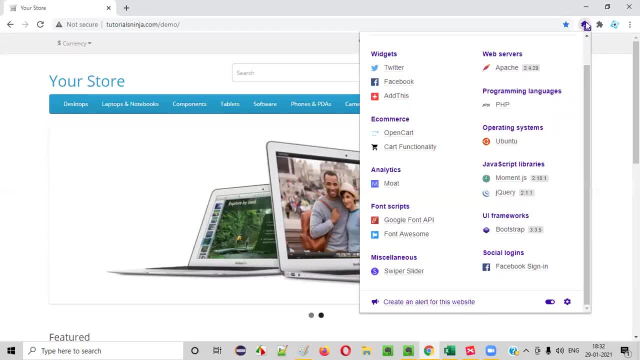 you may not see this big list in the first to go itself. okay, don't think that you'll get this entire list in the first to go. we need to give it some time. you need to browse the application here and there and by the time this add-on will gather all the information from your application. okay, 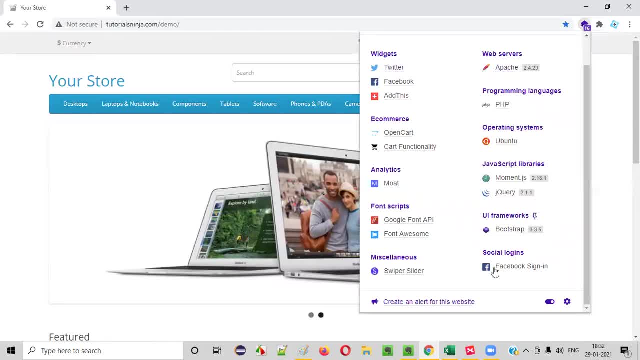 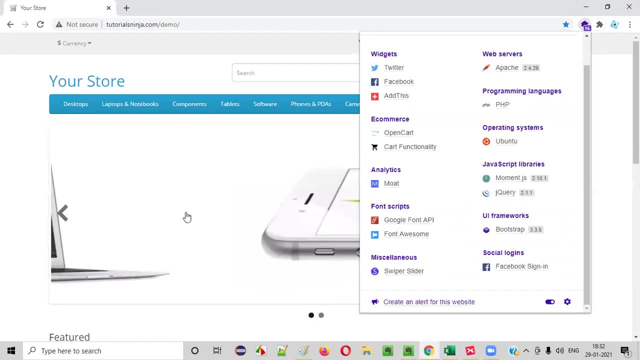 it will take some time for this ad on to show. initially it was showing me only two items now, later it was showing some 10 items. now it's showing some 16 items about this product. guys, okay, this list is building up slowly, slowly, slowly, okay. so the more the time you give, the more the time it will take to analyze this application. 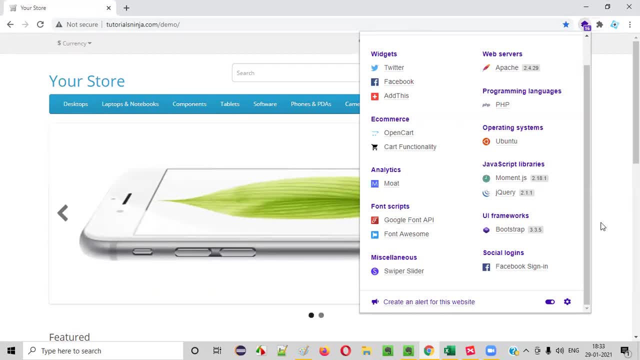 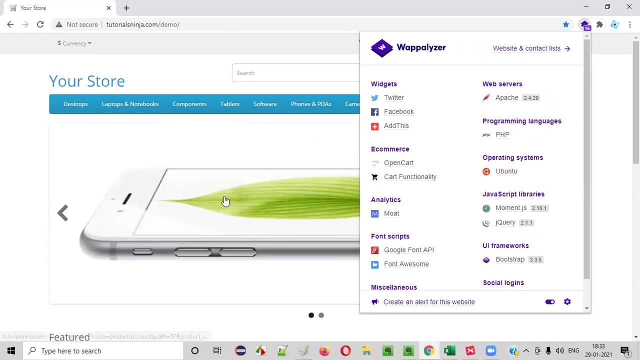 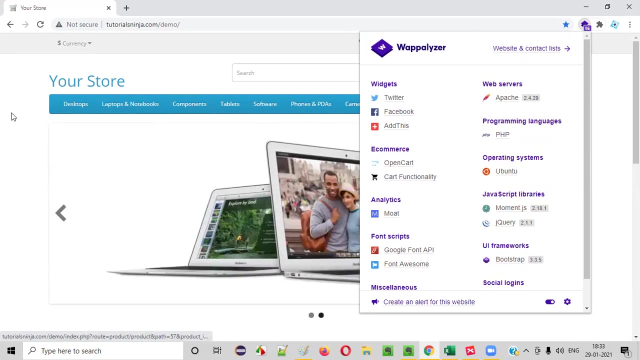 and give you the list of technologies that are used for building this application. fine guys, anyhow, let's find out few important details that we can find about this application in terms of security. so which programming? this is all about security. right as before we perform security, we need to find out or identify which technologies are used for building this application here. 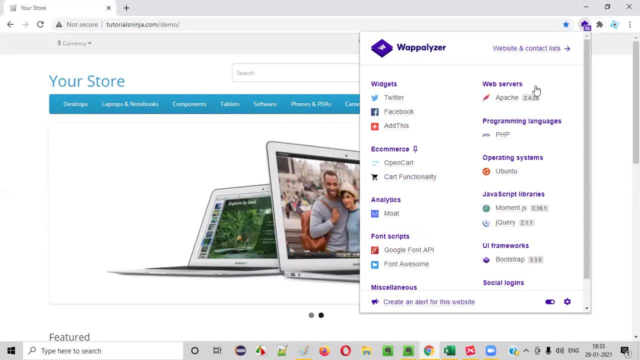 it's clearly stating that php programming language is used. that's one thing. and then second thing is: like web servers, it is using the apache web server. this application is hosted on some server, right? the server is type is apache and with versions, it is displaying as 2.4.29 and in which 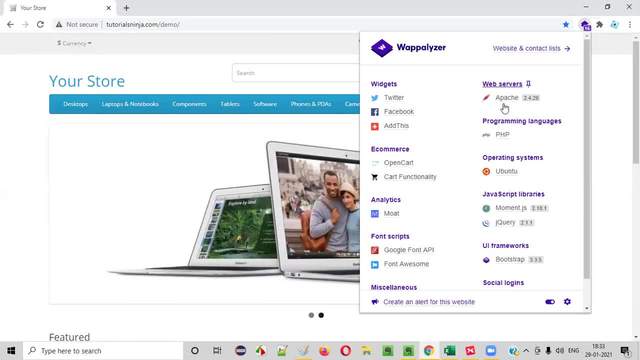 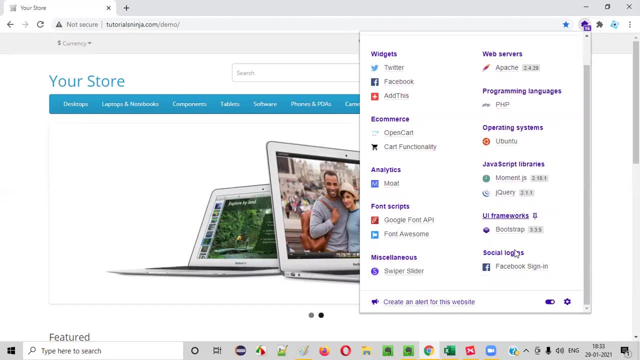 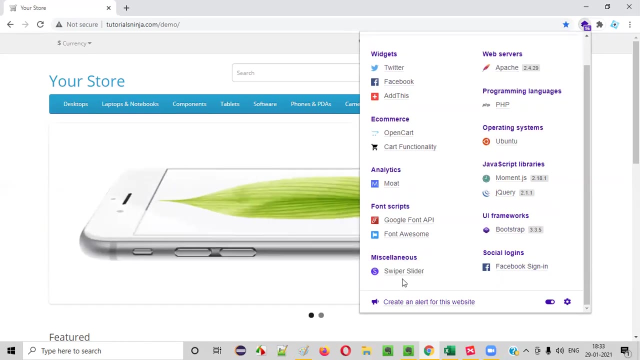 like environment. this particular web server is available. this web server is available in ubuntu linux environment. okay, linux, ubuntu environment. so, like that lot of details we are getting guys like ui framework is like bootstrap, javascript libraries used are like momentjs and jquery. uh, this one, these things are not. 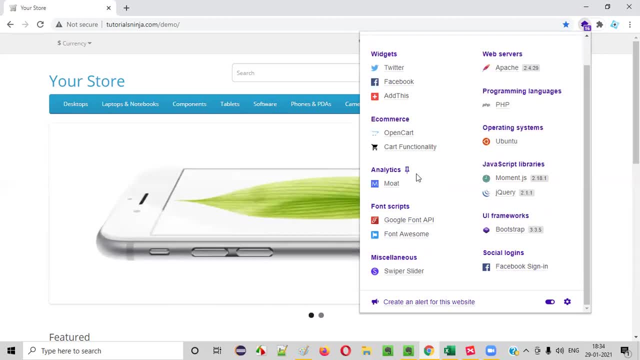 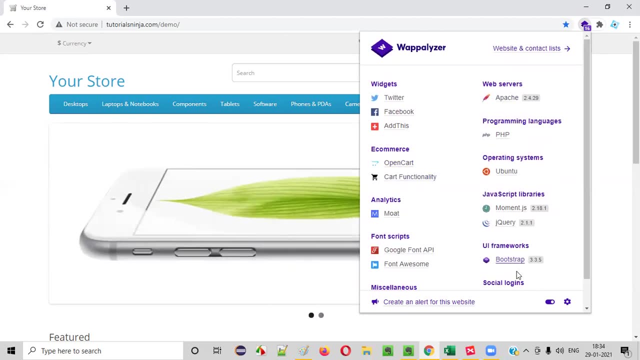 required. anyhow, front front scripts are like google font font- awesome. okay, so it's an e-commerce application from opencart, so this will be enough. guys, this technology will be enough, like web servers, programming languages, operating system, uh, javascript libraries and ui framework. this, this section, is enough. okay, from here to here will be enough. you don't have to. 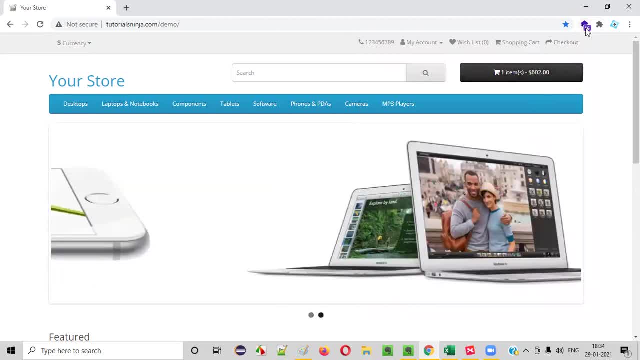 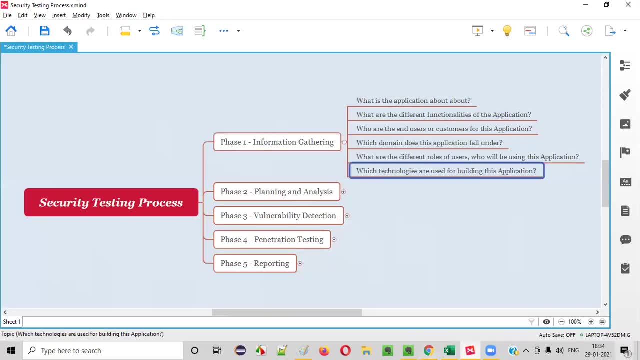 worry about all other the things, other things, okay, this kind of add-ons, guys, we can use, use like vaporizer kind of add-ons we can use for identifying the technologies that are used for building the application. so hope, guys, how to do information gathering right, hope you got some. 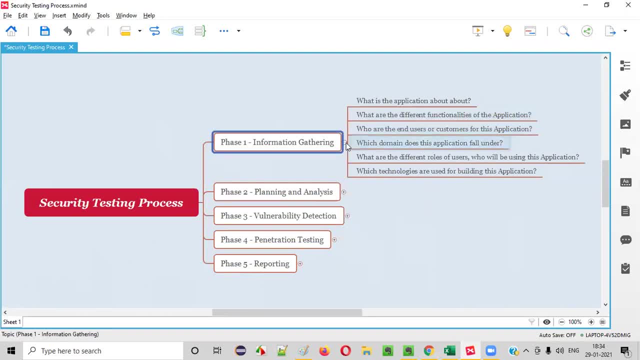 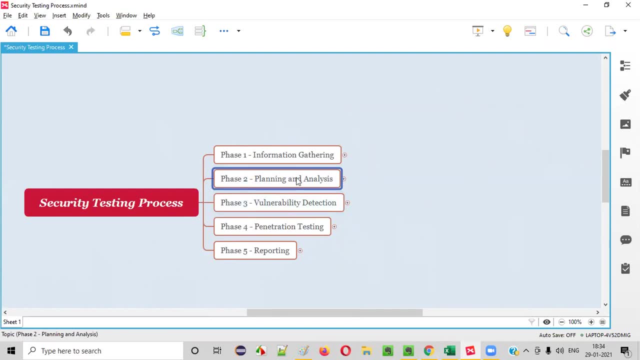 idea like how to do information gathering. once you are done with this information gathering, guys, we'll go to the next phase of secure testing process. okay, that next phase here is: we'll be doing the planning and analysis. okay, we'll do the planning and analysis. what is this planning and analysis? 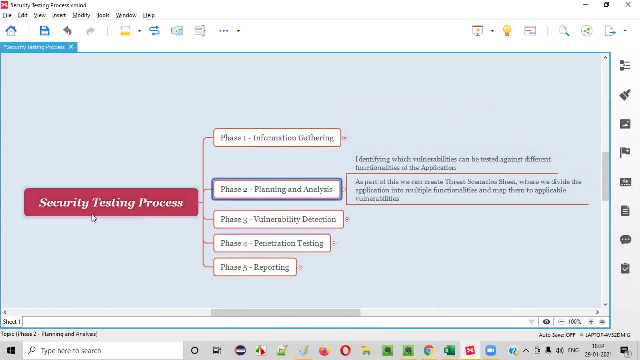 as part of planning and analysis guys, as part of the secure testing process, we will be identifying the vulnerabilities that can be tested across or against the different functionalities of the application. okay, so let's say this application has a lot of functionalities, right? we already gathered the list of functionalities as part of the first phase, right in the first phase itself. 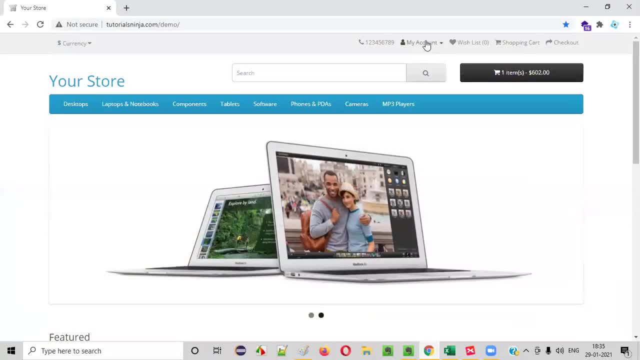 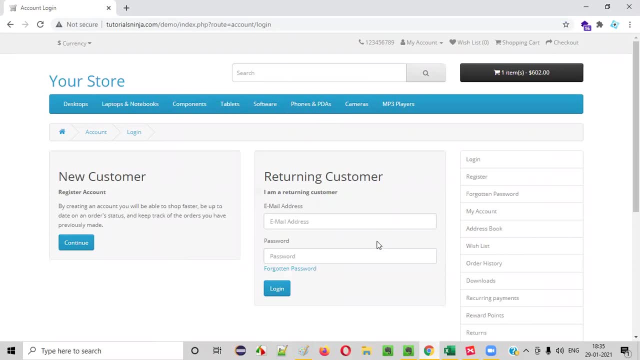 we gathered the list of functionalities available in the application for each and every function. let's say, let's take an example of a one functionality like login functionality- for each and every functionality, which vulnerability we need to test. okay, that's what we need to identify as part of this second phase, for each and every. 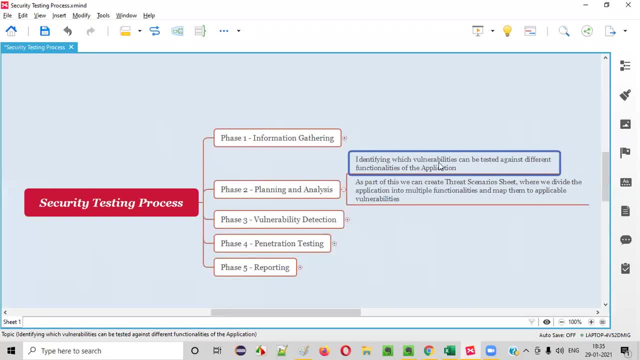 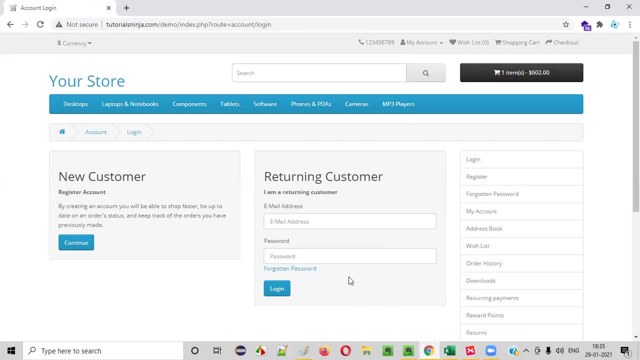 functionality, which vulnerabilities we need to perform testing. okay, so so let's say, if i go to this login functionality guys, i will say that we have to do this sql injection vulnerability. okay, so i'll explain more about the different type of vulnerabilities in the upcoming sessions, guys. okay. 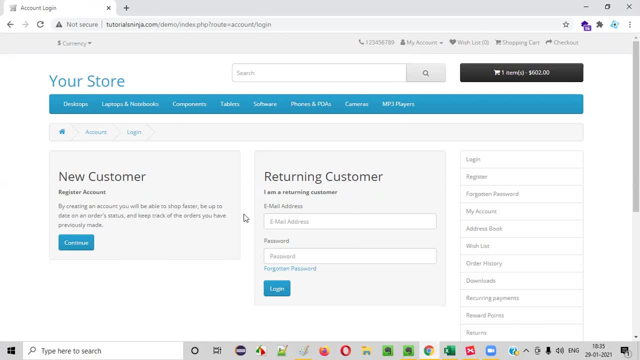 for now, just understand. you already have some idea what is vulnerability, right, security loophole, which categories of security vulnerabilities that we can that are possible in this kind of functionalities we need to identify. okay, at high level. only understand, guys. okay, once we go to the upcoming sessions, it will get more clear for you. okay, you'll. you'll get more understanding of what. 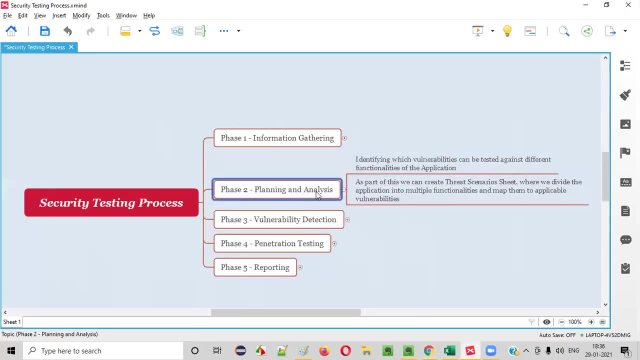 exactly these things are so. so, as part of planning analysis, we are going to uh identify the list of vulnerabilities that we have to perform testing as part of different functionalities across the application. for login functionality, what are the different vulnerabilities we have to perform? testing? for registration functionalities: what are the different functionalities that vulnerabilities? 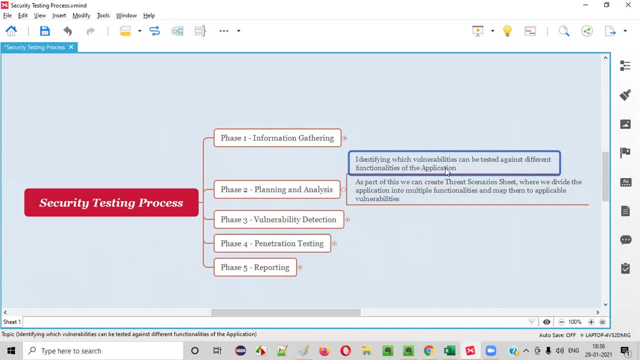 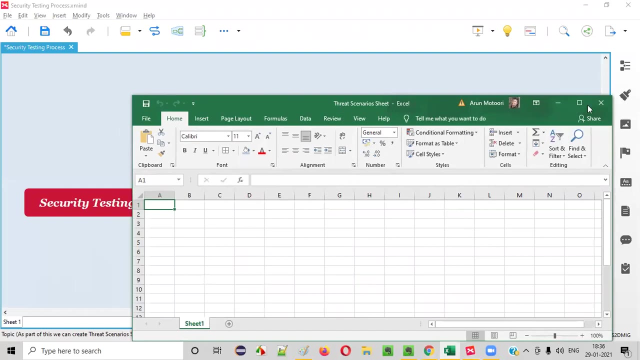 that we have to uh perform uh for identifying them like that. okay, so as part of this identification process, of this vulnerabilities across the functionalities of the application, right, we have to create a kind of excel document, guys. okay, this kind of excel document we have to create. we generally call this kind of document as threat scenarios sheet. okay, so this document is generally. 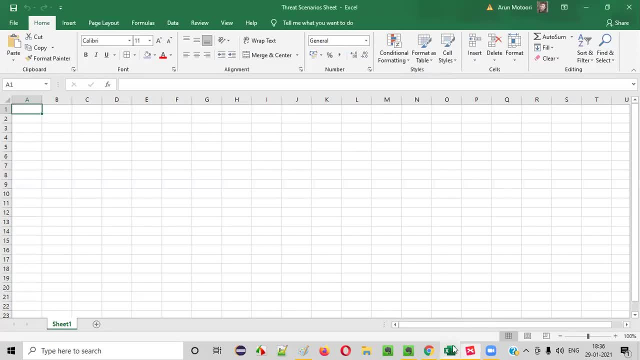 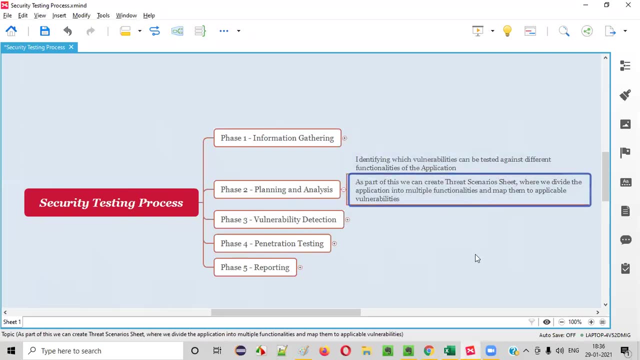 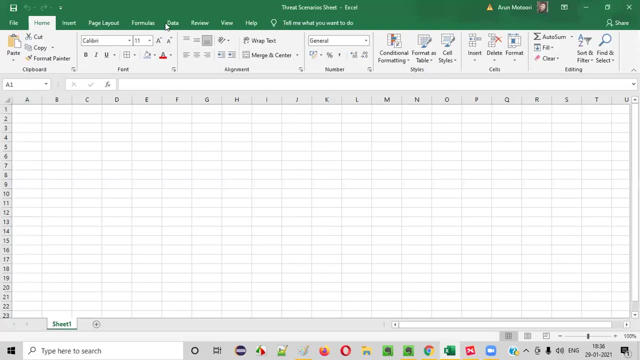 called as this one guys: threat scenario sheet document. okay, this is the document we need to prepare as part of this: uh, identifying the vulnerabilities across the different functionalities of the publication. right, uh, we need to. we need to create this document, excel document with this. it doesn't mean that you have to create. give the same name, guys. this is one of the process followed. 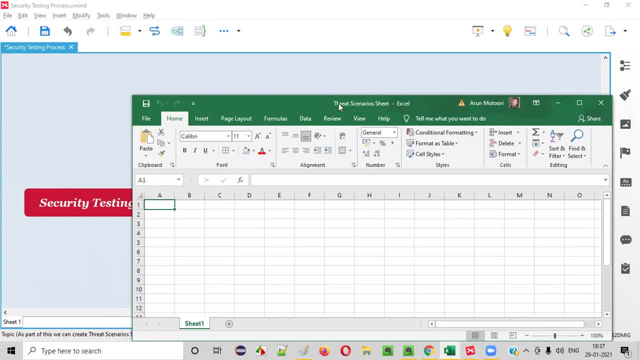 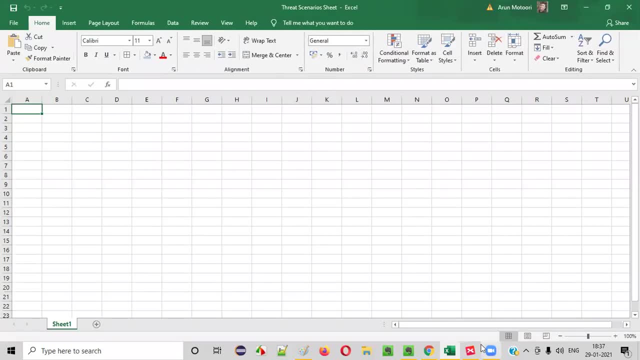 in one of the companies. okay, you may follow different process also. okay, you may follow a different process or different. give some different names for this document. but i am going to explain the intended purpose of this document. why are we preparing this kind of document? fine, why are we? 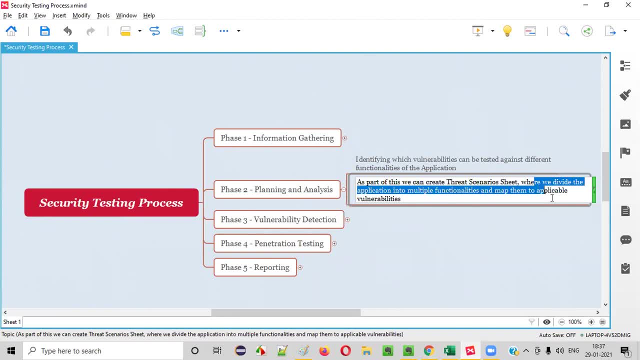 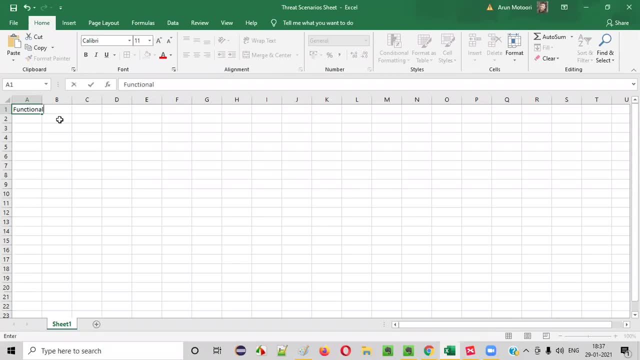 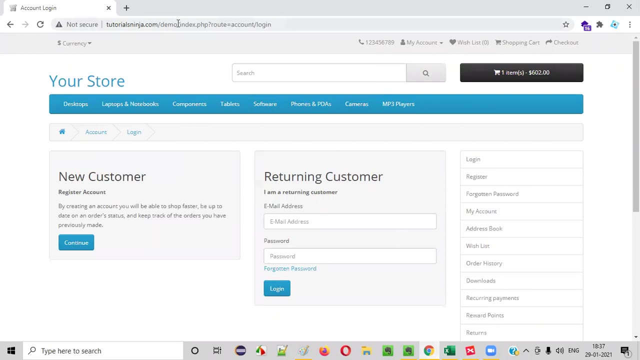 creating this it scenarios sheet. i'm going to reveal for you. so in this sheet, guys, uh, we are going to write something like this: okay, functionalities, functionality. what are the different functionalities we have in this e-commerce application that i'm showing you in this particular video? this particular tutorialcom demo application has different functionalities. 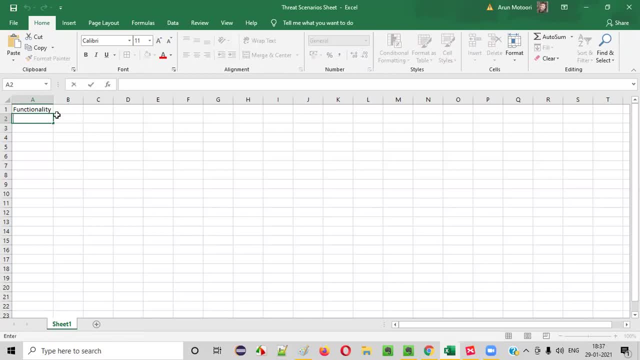 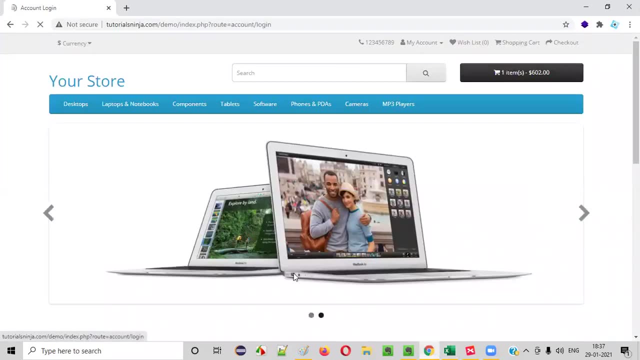 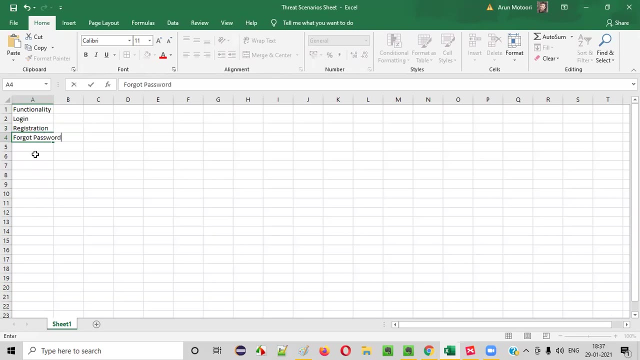 first a functionality. i will write it as login functionality. then we have registration functionality. okay, what are the next functionalities, guys? once we go to the login, we see the forgot password functionality. okay, there's a forgot password, forgot, uh, forgot password. i will write in a short form. you don't have to write in a detailed manner. okay, forgot password. then we have search. 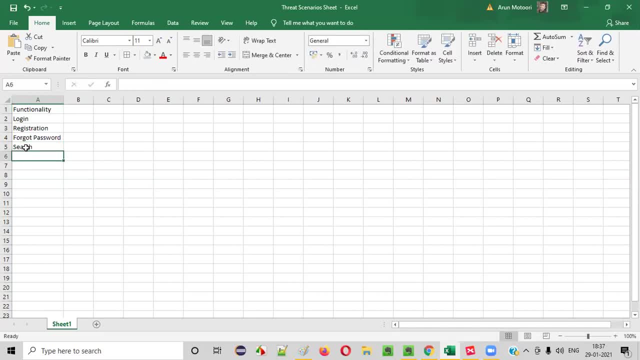 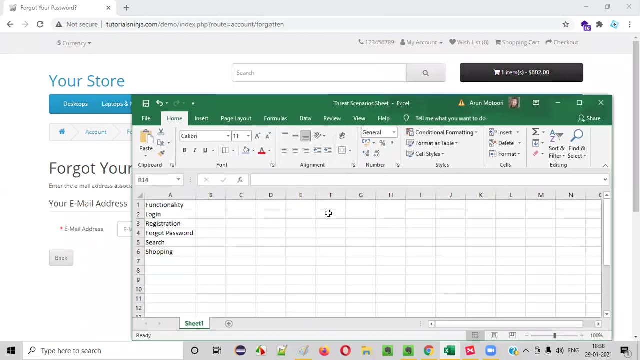 functionality. then, uh, we have, uh, what, uh, this shopping cart functionality. okay, i'm just identifying at a high level. guys, it don't. uh, this is just a high level. this is not the real document that i'm going to show you in the upcoming sessions. guys, we'll create this kind of a detailed document. okay, we'll do a. 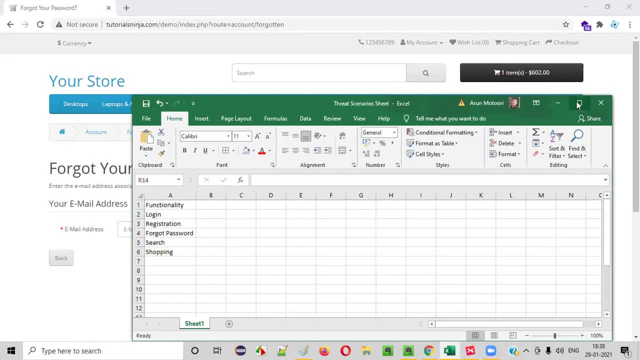 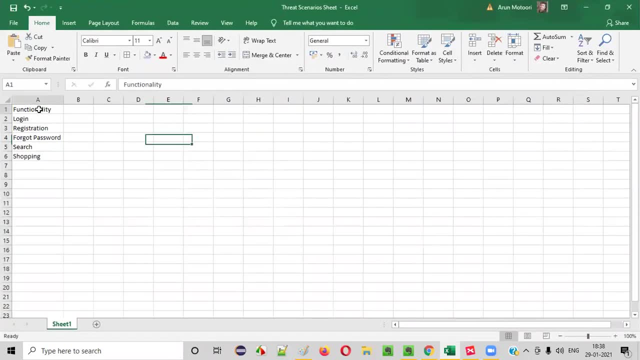 complete live project on security testing where i am going to show you how to prepare the entire threat scenario sheet in detail for a particular project. okay, for now, just we are just understanding the process, that's it. so, like this, a lot of functionalities will come, guys. okay, i'm not. 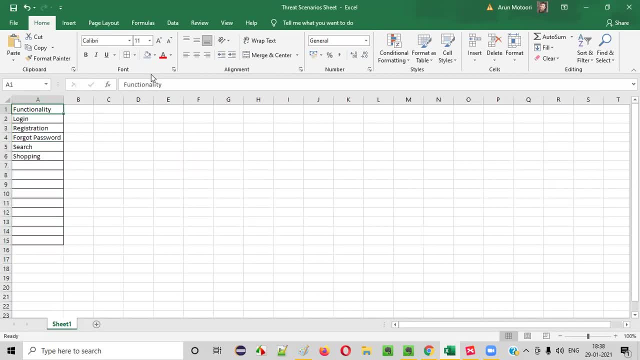 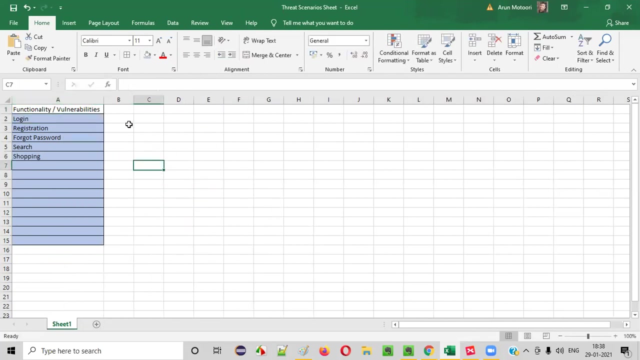 listing down all the functionalities here, so let me just give some kind of colors and all so that they will look good. okay, so there is a function list of functionalities on the right side. guys, on the on this right side, you have to say functionalities by vulnerabilities, vulnerabilities like this. okay, we have to write like this and here: 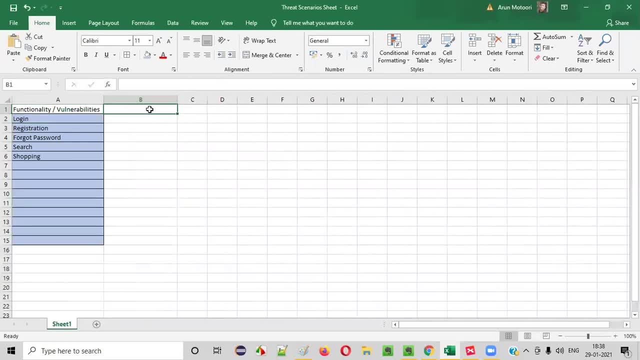 for each and every functionality, what vulnerabilities we are going to check. okay, anyhow, irrespective of which function, which vulnerabilities we have to? uh, we are going to perform testing for these functionalities. we'll just list down all the vulnerabilities here. okay, so one type of vulnerability is like sql injection. 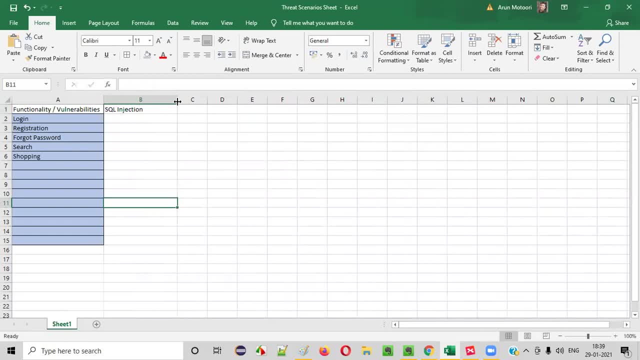 uh. then we have other thing like: uh, cross-site scripting, xss. i'll say xss for now. okay, we have cross-site scripting, sql injection and many other. are there, guys? okay, many other vulnerabilities like: uh, i'll simply okay, without wasting any time. i'll simply say: vulnerability three: okay. 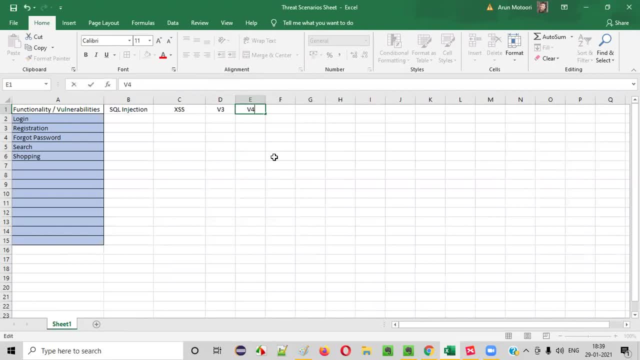 just assume that these are the names of the different vulnerabilities that are possible. so how many vulnerabilities that we can generally test for all the functionalities? right, that vulnerability list we are providing here here list of functionalities in the application, here list of vulnerabilities we can test. okay, like that. so v3, v4, like all the vulnerabilities that are generally. 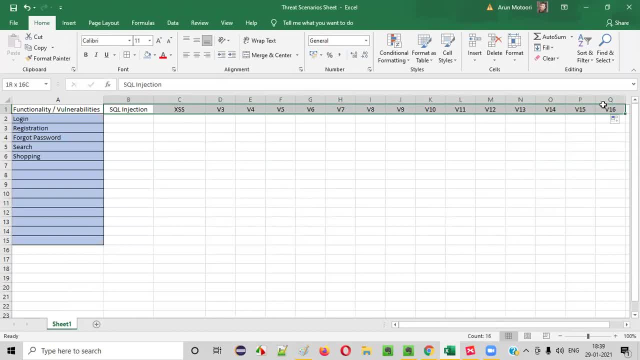 tested as part of secure testing will be provided here, so i'll just color it in a different way. uh, i'll just give some color. sorry, i'll just select a different option. that's fine. uh, for this, i'll just give a this color. okay, so here, functionalities by vulnerabilities: i'll give a different color. 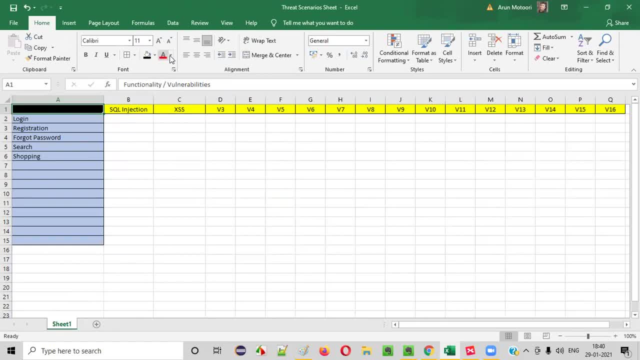 i'll just give black color and then i'll give the font as white so that you can see like this: okay, so now these are the boxes we have. so you are just getting idea, right? uh, like, how does it? uh, how does this particular threat scenario sheet will look like on the left side. we'll have 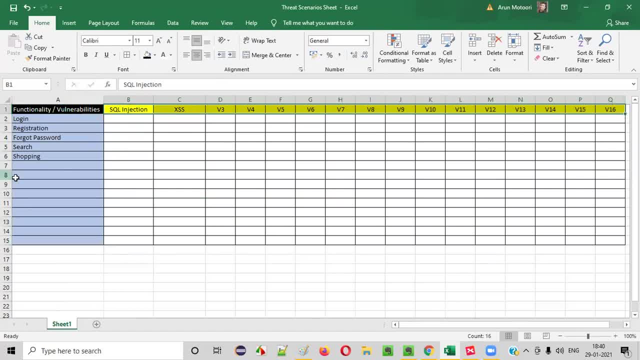 a list of functionalities. on the right side we have the list of uh vulnerabilities- okay- and that we can test as part of this, functionalities. let's say, for login functionality, sql injection is applicable. okay, applicable. i'll write applicable. i'll write simply: applicable. this is applicable or not? okay, we are not testing it. 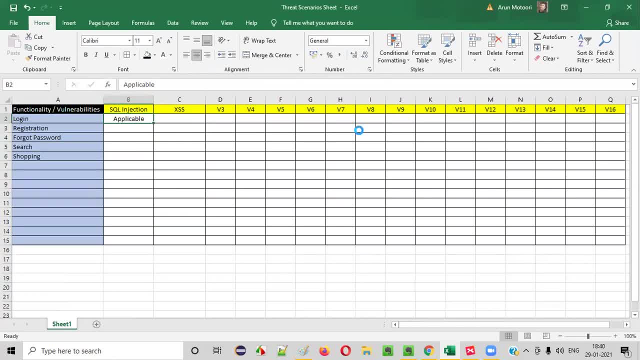 guys, whether it is applicable or not, we are just mentioning: okay, let's say this is not applicable. randomly, i'm writing: guys, this is not the exact data, this is not the correct thing, i'm just, uh, randomly writing something as applicable, something is not applicable, like that, okay. 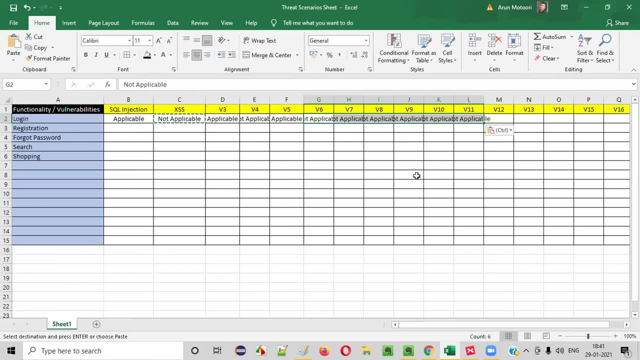 like this not applicable, this is not applicable, these are all not applicable. okay, like that. i'm just randomly writing so just to show you how the templates, how this particular template, will look like. okay, fine. so similarly, uh, we'll be writing for remaining also not applicable and all and uh, let's say for this thing, registration, let's say: 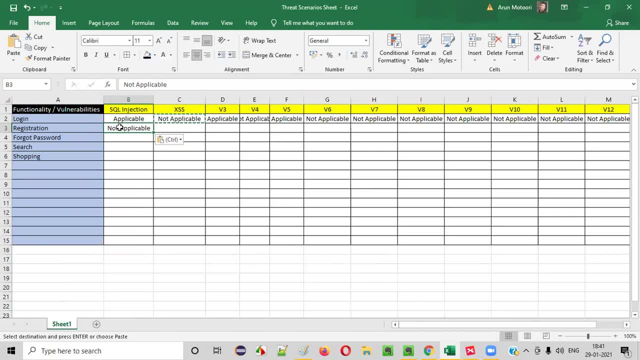 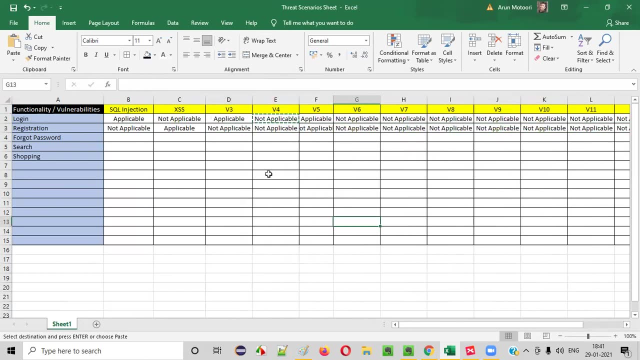 this is not applicable. okay, this sql injection is not applicable for registration. xss is applicable for registration, like that. okay, remaining or not applicable. let's say remaining, all are not applicable. okay, fine, so like this: guys, we will be filling this entire form. okay, we'll be filling this entire uh form. 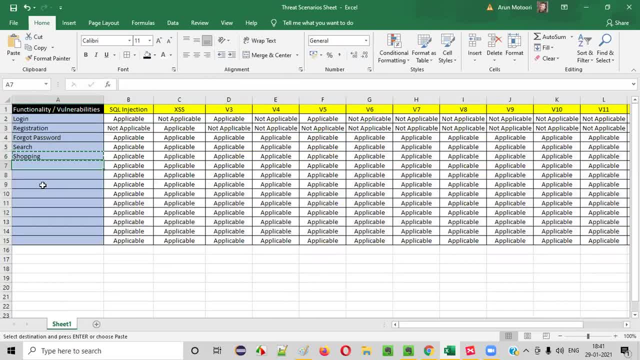 like this: uh, this side, all the functionalities will be there. okay, i'm just filling up the form. let's assume that these are all the list of functionalities in the application and these are all the different vulnerabilities that we have to perform testing as part of this across different, different functionalities. this is a kind of 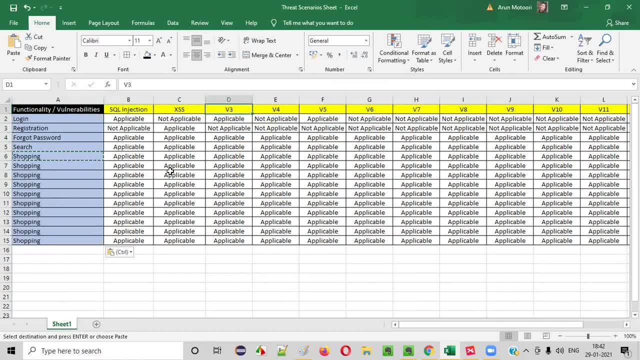 like mapping right, mapping between the functionalities and the. this document is like a mapping between the functionalities and the vulnerabilities for this login. which vulnerability is applicable? like that: okay, if it is applicable, we have to perform testing in the coming phases. like that: this is just a template, guys. okay, so this kind of sheet we need to prevent. 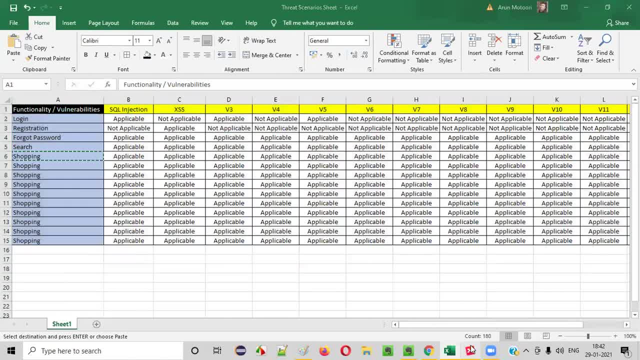 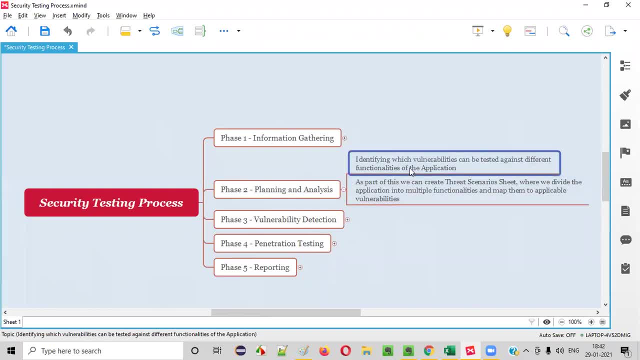 this kind of sheet we need to create. in which phase, guys? this kind of, uh, threat scenario sheet we need to create in the planning and analysis phase. okay, the planning and analysis phase. we need to identify the list of functionalities that need to be tested in the application. 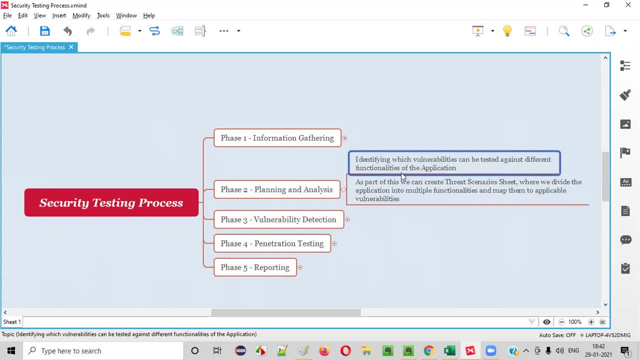 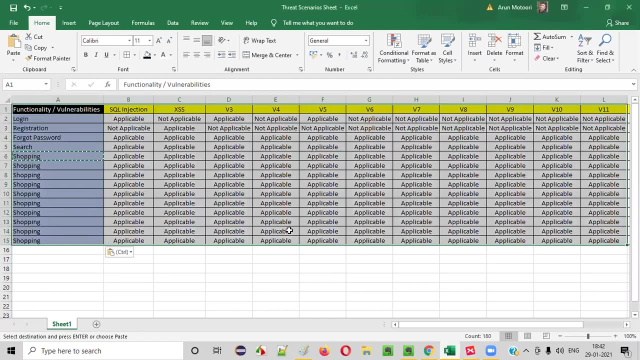 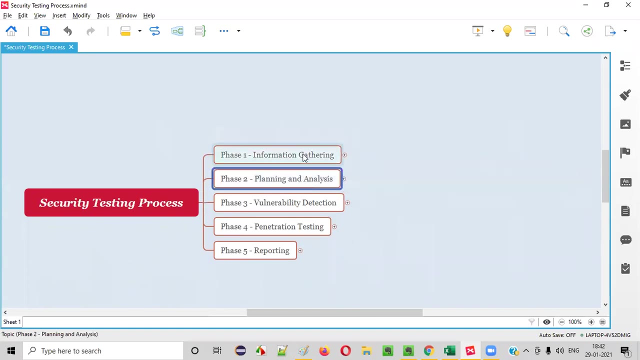 and on the other side, we list down all the vulnerabilities that can be tested across these different functionalities of the application in this particular threat scenario sheet. okay, the sheet will look something like this: fine, so this is just a creation of the sheet case. nothing much. this is nothing but the planning and analysis phase. now let's go to the next phase. 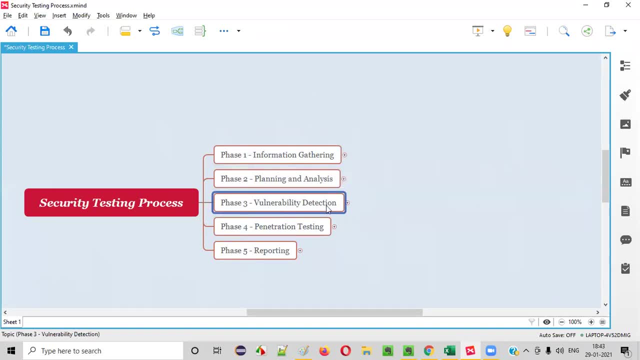 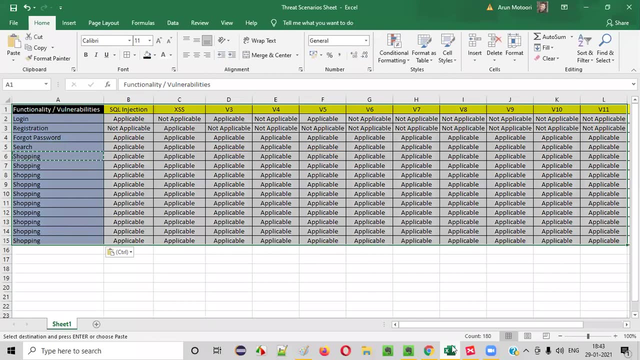 now let's go to the next phase, that is, vulnerability detection. okay, the next phase is vulnerability detection. in this phase, this vulnerability detection phase, what we are going to do here is we are going to start testing this. okay, as part of vulnerability detection, we are going to 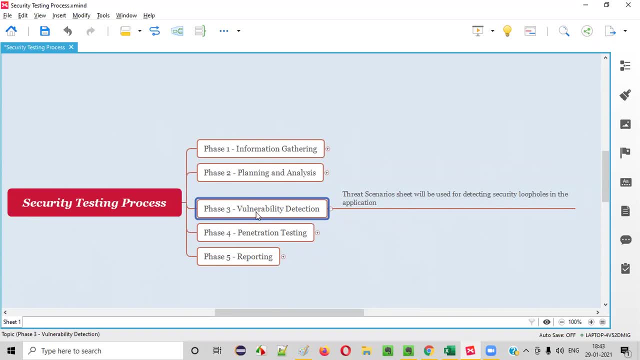 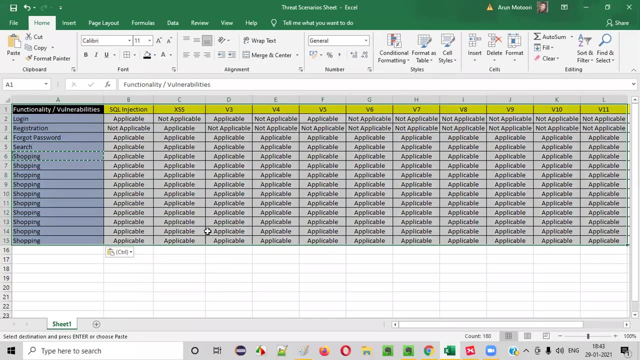 okay, it's a vulnerability assessment process. you can see. okay, the third phase, like vulnerability detection or assessment, where we really perform testing. we will put this particular sheet before us. okay, this particular sheet is created. in which phase, guys, in planning and analysis phase, we created this sheet. now we will follow this particular sheet and then we are going to start. 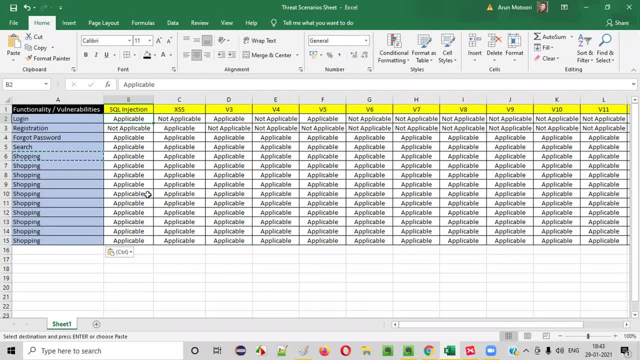 testing this? okay, so we will follow this sheet and perform testing. till now, we didn't perform testing, guys. okay, so how do we perform testing using this particular threat scenario sheet? okay, we'll be using this sheet for starting the testing. so we'll start here, guys. sql injection and. 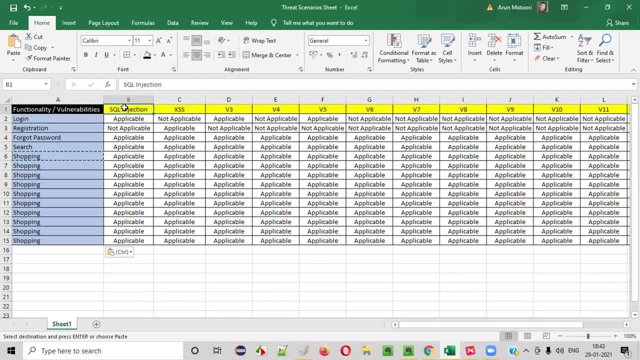 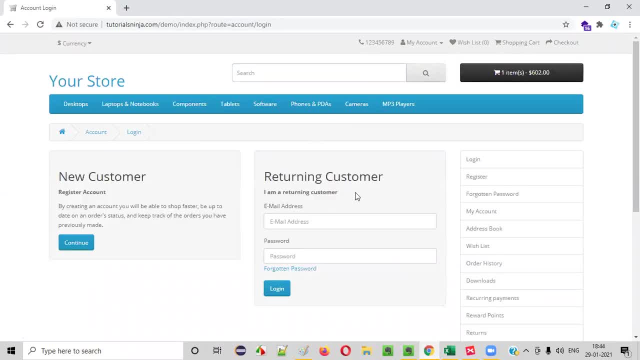 first we'll start with the login functionality and first vulnerability type is like sql injection. we'll see whether this sql injection is applicable for this login or not, so we'll go to the login page. okay, in this particular application, we'll go to the login page and we'll do some sql injection. 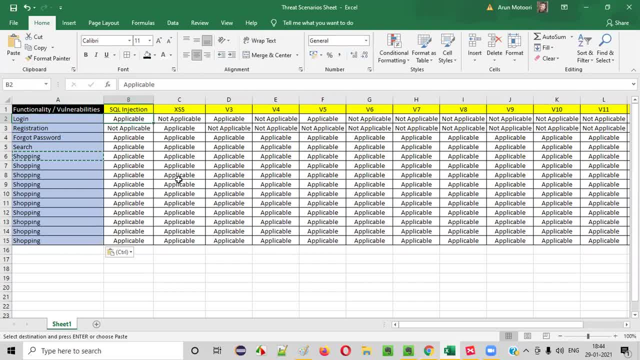 kind of stuff here. okay, this particular thing is applicable for this login, right, so we'll perform the sql injection as part of the security tester and then, if there are no issues, okay, if there are no vulnerabilities- sql injection vulnerability is identified in this login functionality- we'll pass it. 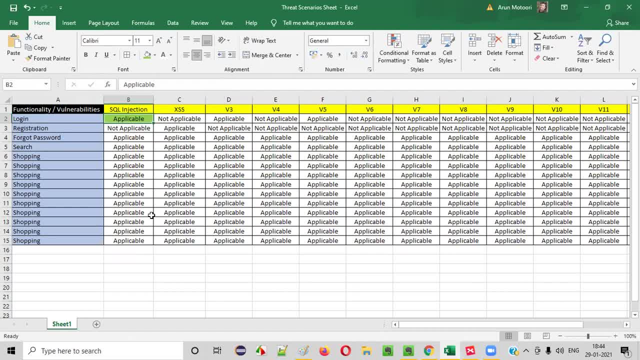 we'll simply pass it, mark it as pass. okay, now this is not applicable, so you'll not be testing. not applicable, you will not be testing. then the next one. let's say, another vulnerability is there which need to be performed for this login functionality, that is, v3 vulnerability. for now, the dummy vulnerability. so again, we'll go to the login. 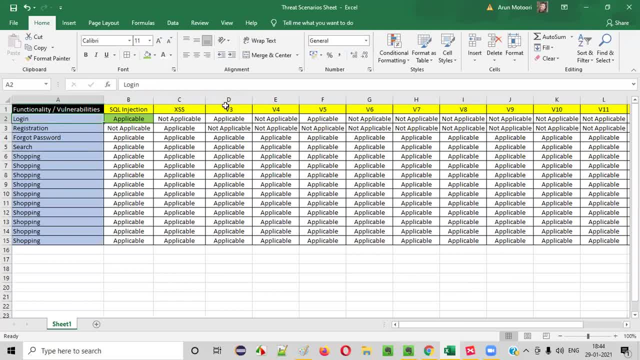 page and check whether this particular login functionality is having any security lo loopholes in terms of this v3 vulnerability. okay, let's say you identified some defects, you identify some vulnerabilities which are coming for this category of vulnerability type for login functionality. so you have to fail it right. you will fail it like this, like this guys. 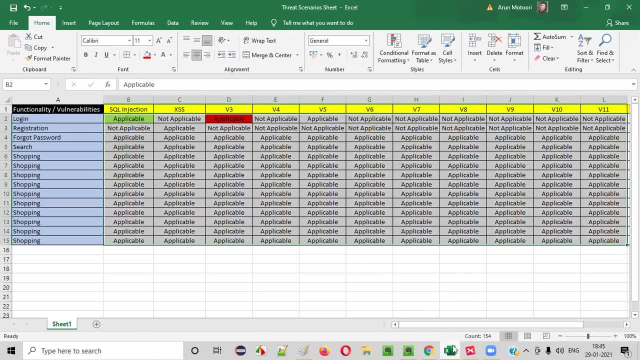 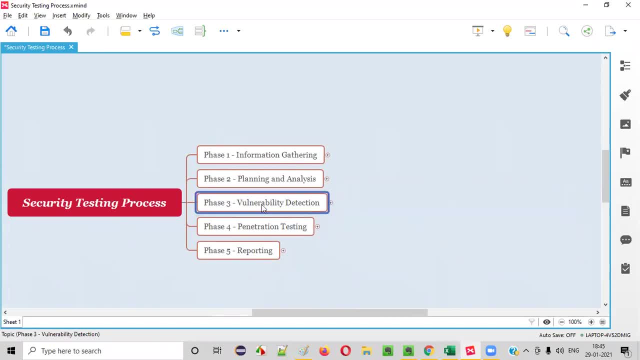 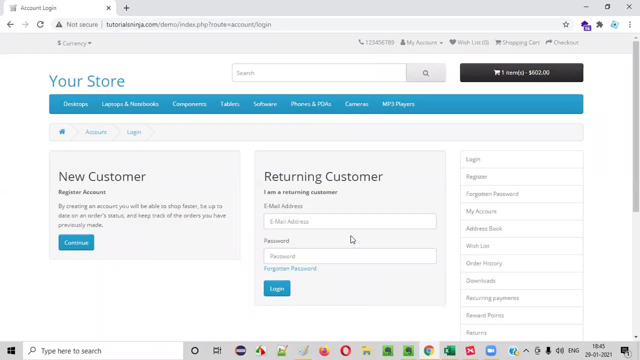 you will be testing this. uh, okay, you'll be using this particular sheet for testing, performing the security, actually security testing, as part of this vulnerability assessment. okay, this is the third phase, guys. in third phase, we will only identify whether this particular functional areas of this application are having any security loopholes or not, that is, security vulnerabilities or not. okay, that is a. 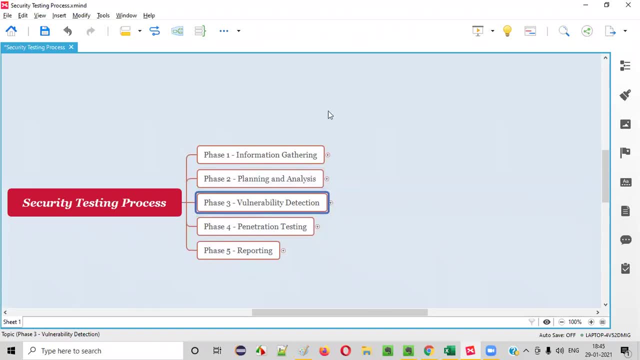 vulnerability assessment. i explained about more about the vulnerability assessment in the previous sessions. guys, you can go through that if you have any doubts. now, once the vulnerability detection is done, then the next phase will come, where we perform fourth phase. guys, okay, fourth phase of the security testing process, where we will be performing the penetration. 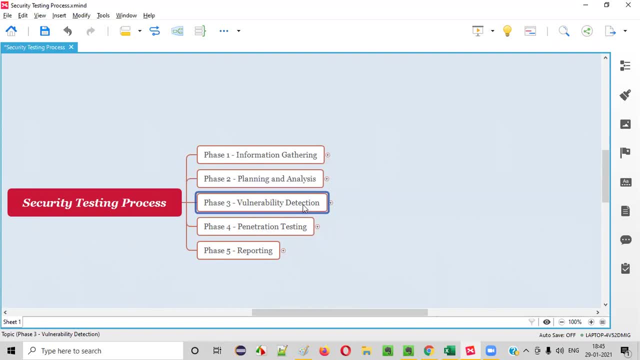 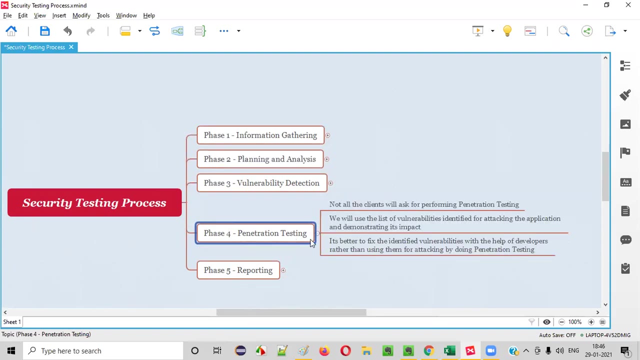 testing here only identifying whether the functionalities have this vulnerability problems or not. okay, any security loopholes are there in the application or not? we are just finding it out, okay. but here in penetration testing, guys, it's a different thing. okay, penetration testing is a different thing, where we will use this identified vulnerabilities and try to hack the application as 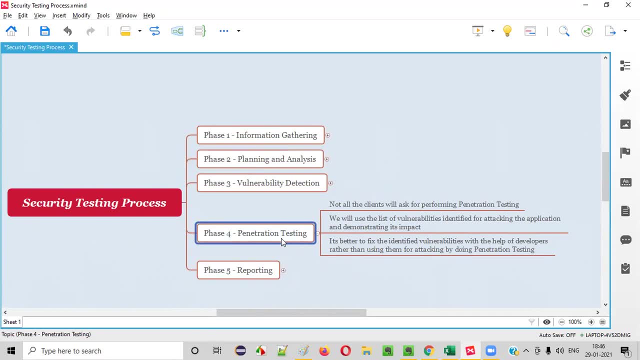 the attacker does okay. okay, it's a kind of ethical kind of hacking. you can say, guys, where you will be performing this penetration testing by behaving like an hacker, okay, but uh, your intentions are good- only just to see, like, uh, whatever the security loopholes or vulnerabilities you identified as part of the 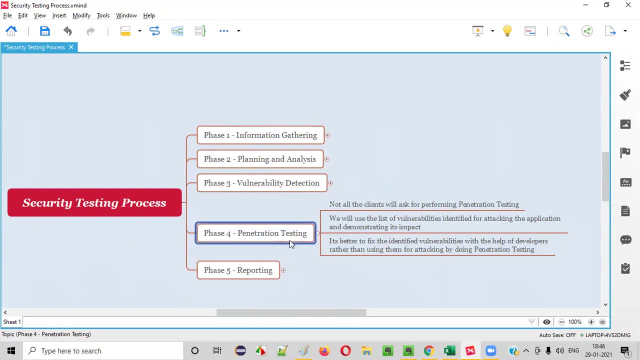 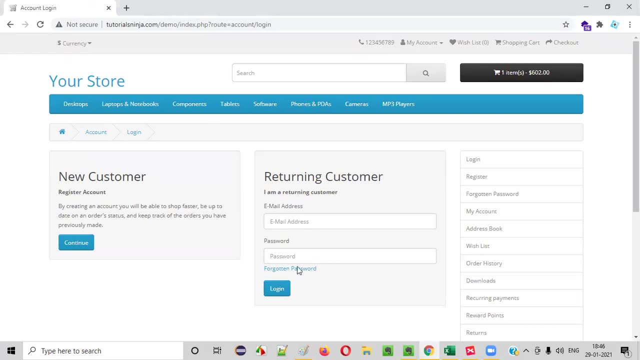 previous phase what kind of impact they are causing. let's say, because of this sql injection. okay, because of this sql injection. let's say, the user is able to log in. okay, without even having the permissions to log in, user is able to log in. let's just go to the leading data point. okay, let's just. 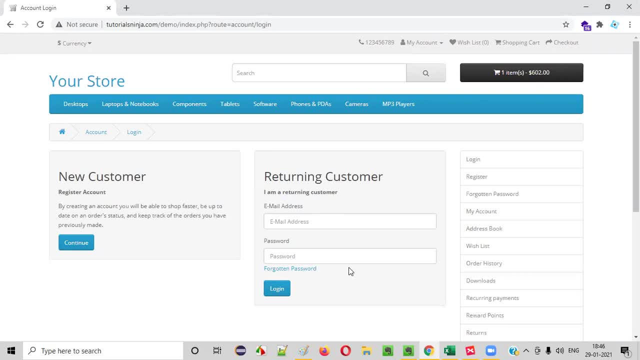 that's why we will be looking at the system, looks at these instructions. okay, to take the action flow. let's say, okay, without having the proper credentials, user is able to log in such kind of sql injection. let's say, okay, by using the sql injection, this is uh, this may be possible where. 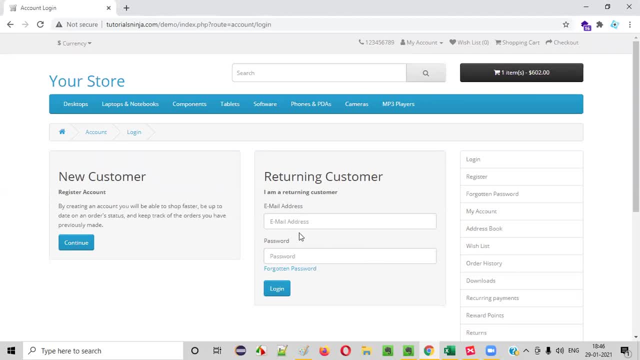 attacker can use sql injections to find out the way, without even having the proper credentials, he can log in. so what is the impact here? the attacker is able to hacker is able to log in, right. so such kind of things. sometimes guys like attacker can go to a level where he can destroy. 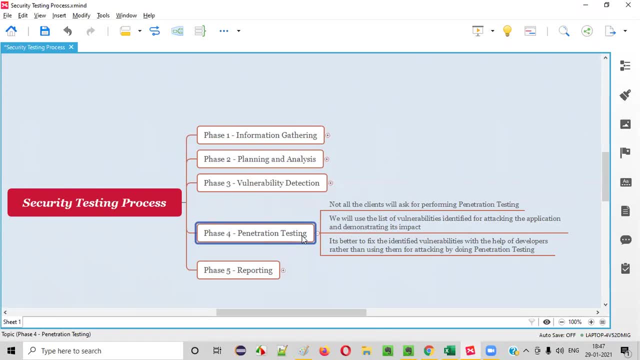 your db. completely okay, he'll log into the application, he'll access the db, he'll take the complete db into his control and he will delete the particular, all the data in the db. uh, okay, or he can copy all the data from the db. whatever it is, whatever is possible, right, that we can perform. 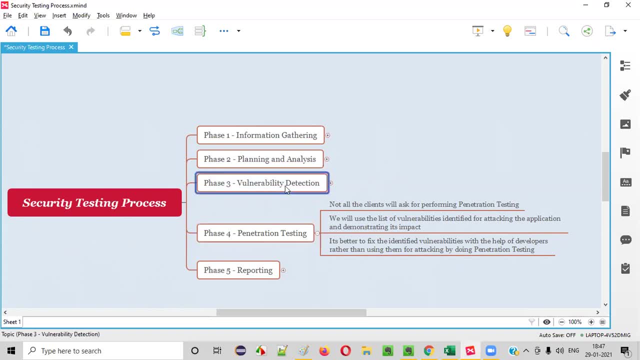 okay as penetration testing. once the vulnerability is identified, to what extent this vulnerability can be utilized is part of the penetration testing. but, guys, there is a clause. the thing is, you can't use sql injection to find out the way without having the proper credentials. not all the clients will ask you to perform this penetration testing, so whenever you get an 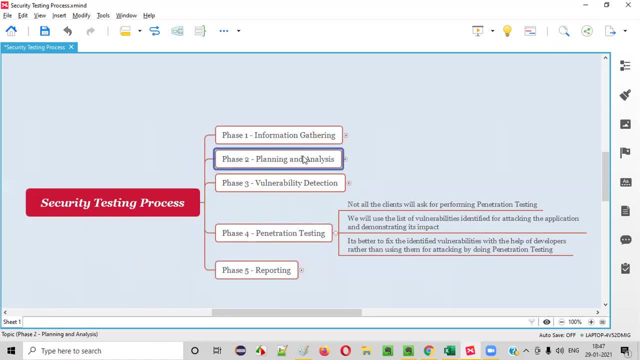 application for performing the secure testing. you'll first start with the information gathering, planning analysis, value, value, where you create that particular sheet, threat scenario sheet. then you will uh start identifying, i mean you will start performing the vulnerability assessment where you will detect all the vulnerabilities in the application across the different functionalities. 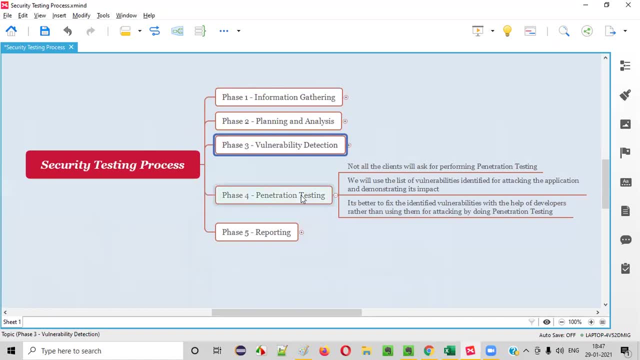 of the application, then you'll go for the penetration testing. but penetration is not, uh, compulsory, guys. okay, before you go for the penetration testing, you will need to perform penetration testing. before we perform penetration testing, we need to take necessary permission from the client. okay, because there is a problem with the penetration testing. so because 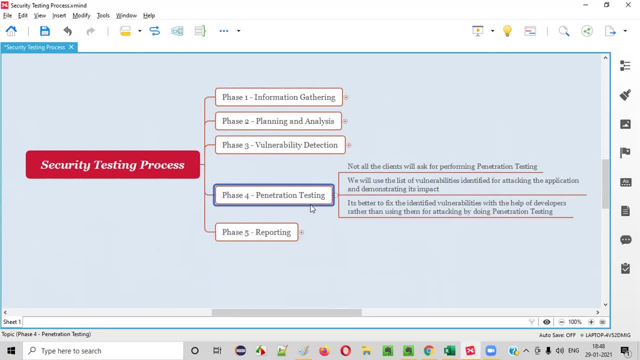 the application may go down or you will destroy the db of the application because, client, there may be some sensitive information in the application and that client has not notified you or whatever happened, right? so when you perform the penetration test, you cannot get the data back. okay, once you. 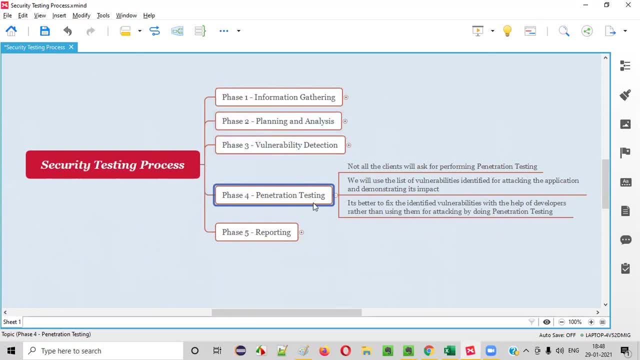 destroy the db by using some penetration testing techniques. then if the client tomorrow ask you like to restore the db, you can do that. but before that you have to do the penetration testing and you cannot do it. okay. so such kind of problems are there. we need to educate our client that, okay. 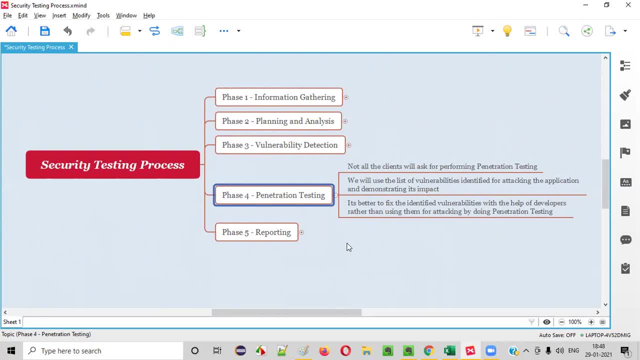 penetration testing will cause all these kind of damages. are you okay with this? and uh, what will happen if the db will really get deleted and all those stuff? everything you need to discuss with the client guys. okay, before you perform penetration testing, take necessary permissions from the client. 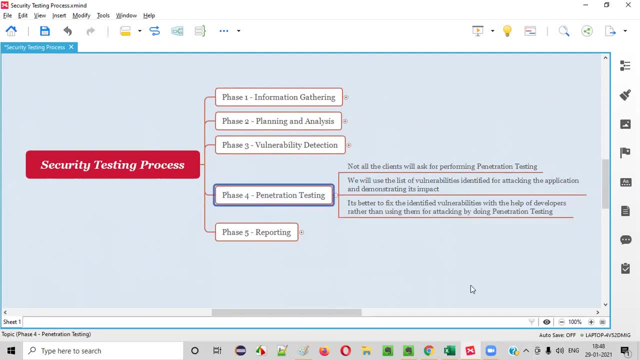 and also, guys, not all the clients will accept for this penetration testing. only few clients, like three or four out of hundred clients, will accept for the penetration testing. and even they accept. guys, it's your duty to, it's your duty to educate the client about the consequences of performing the. 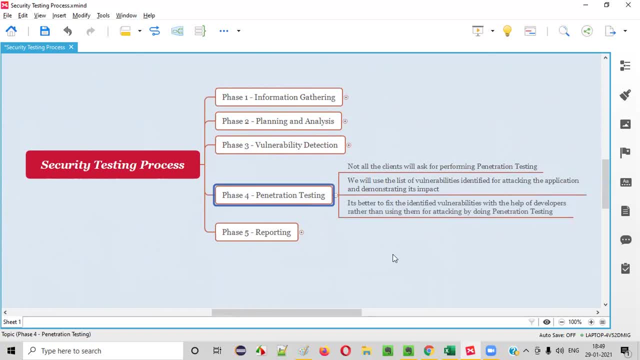 penetration testing because that may lead to some loss or damage of the application. okay, so before you perform the penetration testing, you have to cross check all these things with your client. fine, and also guys. the final suggestion is like: uh, yes, as as a part of penetration testing, we can go to. 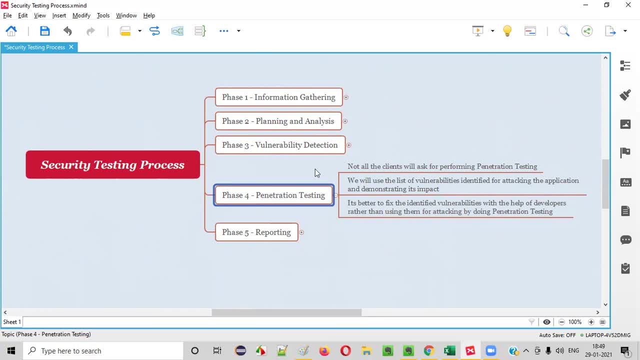 the level of extent where we can damage everything in the application. right, if there is a possibility of uh damaging the things we can damage. but, guys, it's often uh good advice, like uh it's. it's rather a good thing to fix the identify vulnerabilities by sitting with the developers rather than attacking it as a penetration tester. 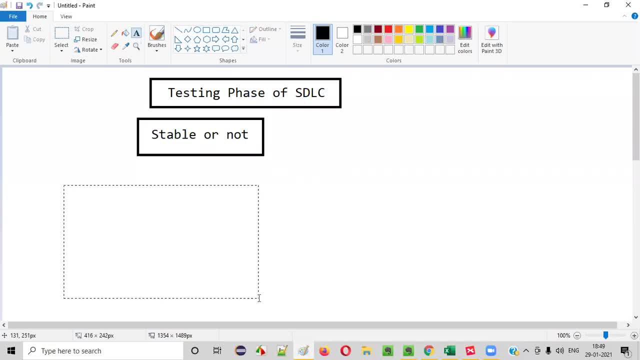 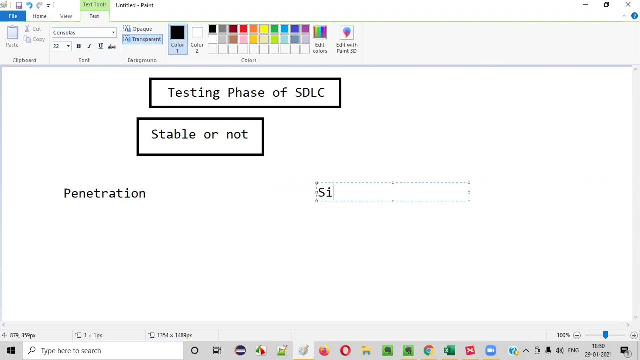 okay, so instead of instead of doing the penetration testing, instead of doing the penetration testing and seeing what level of impact or damage the that can that a particular vulnerability- that is, identifying the application- can cause to the application, right, rather, you can sit with the developers. okay, you can sit with the developers and get it fixed. this fixing of the defects is better than 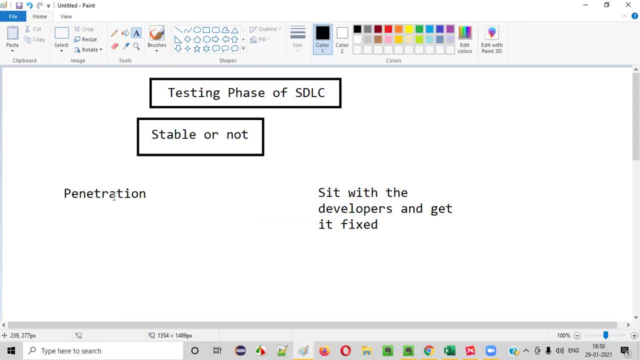 penetration guys. if the defects got fixed, why do we have to go and check with for the impact guys? okay, if you are able to impact, like educate this particular thing to the client, then you can avoid this penetration testing. okay, you can avoid this penetration testing and more. you can focus more on. 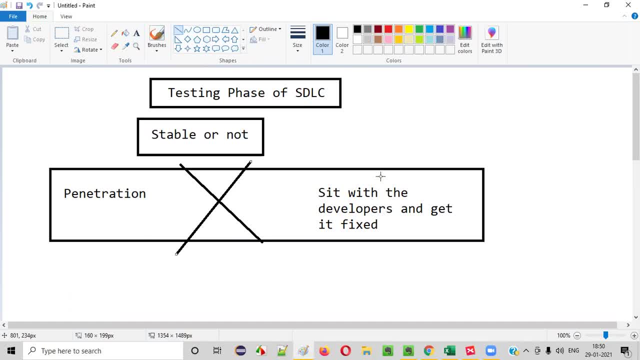 vulnerability assessment and getting the fixer the security problem fixed from the application. fine, so this is a better uh thing that you can educate to the client, but if the client uh really want you to perform penetration testing, then go ahead after after you uh did all your efforts. 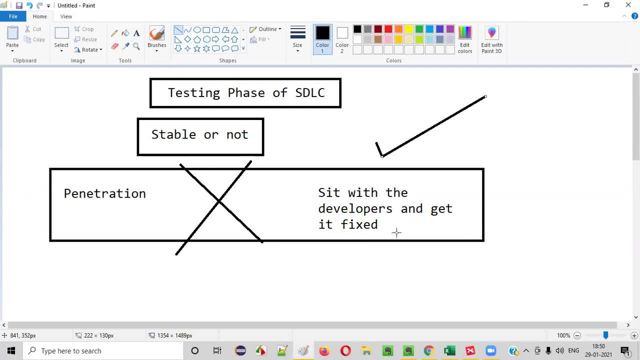 in educating the client that, uh, we can identify the vulnerabilities, we can get it fixed and, uh, if there are any other things, uh, that developer is not understanding, then you can go for penetration. such kind of understanding if you give to the client right, then that will be good. 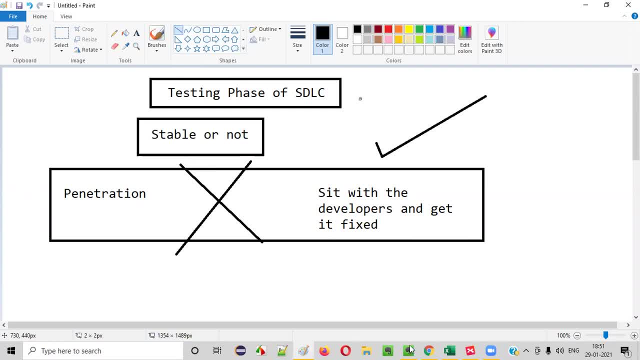 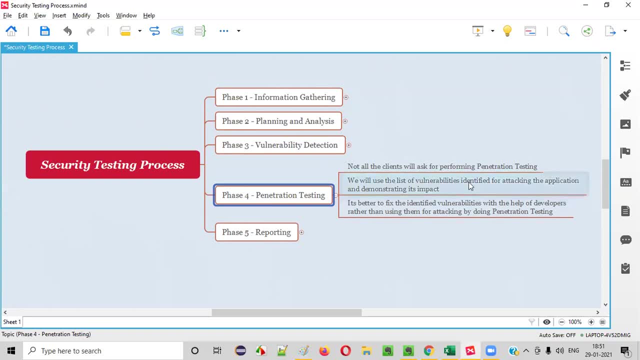 but if the client is not listening, then if there is no way, you can perform this. so this is part of the fourth phase of the security testing process. we can perform the penetration testing. uh, as i explained, right, not all the clients will go for this kind of option. 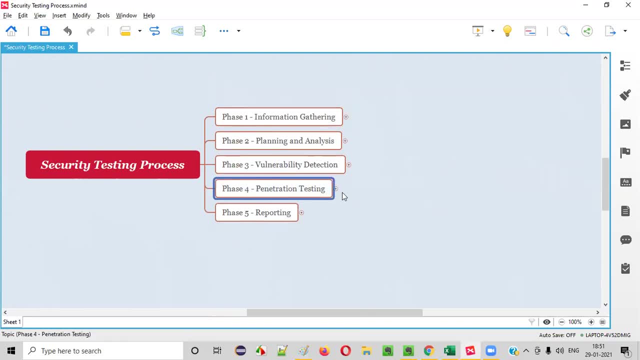 and if a client goes, it's our duty to educate the client. that duty to educate the client that penetration testing is not always required, okay, so we can get the fix defects fixed, and then, uh, later we can do- or it's not at all required- such kind of things we can educate with the client. 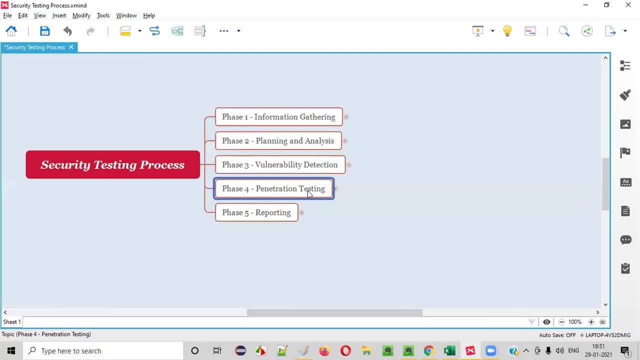 until and unless there you get a proper reason where you have to test the client. yes, i think that's the one thing to keep in mind. you can certainly perform the penetration testing. you should not be performing the penetration testing, guys, so otherwise the client is insisting, then you can do. fine. then the last thing, guys. okay, after all these four phases are done, the last phase. 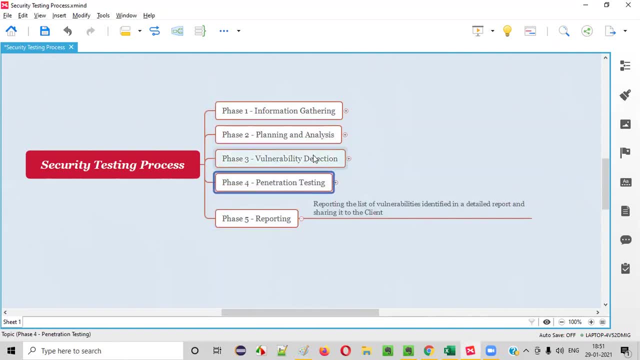 is about reporting. so, whatever the testing you did as part of vulnerability assessment or penetration testing, right. whatever the testing you performed, right all these things, you need to create a report, a detailed report you need to create, with a list of vulnerabilities, their names, their descriptions, their steps to reproduce a lot of stuff, guys. okay, screenshots, videos, what have you? 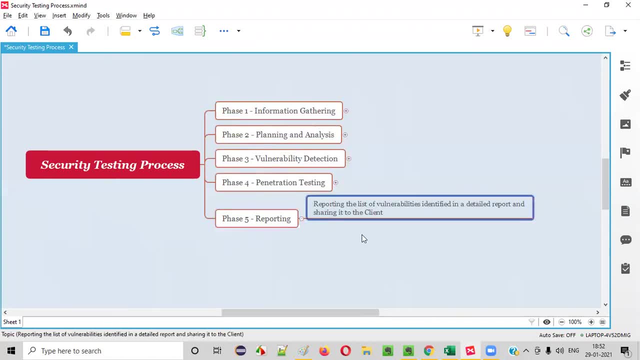 it is as a proof. whatever you can provide, okay, whatever the impact that the vulnerabilities can do all those stuff with your knowledge as a security tester, whatever the knowledge you gain, right with that knowledge, you are going to create a detailed report at the end of the project, okay. 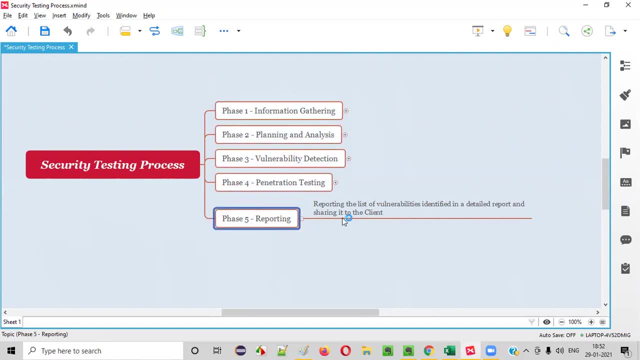 during this phase, at the end of the cycle or project, you will be creating this kind of report and sharing this particular report with the client. okay, i'll be showing you. i will be showing you how to create a report in the upcoming sessions, guys. okay, for now i'm just uh, explaining at a high level. 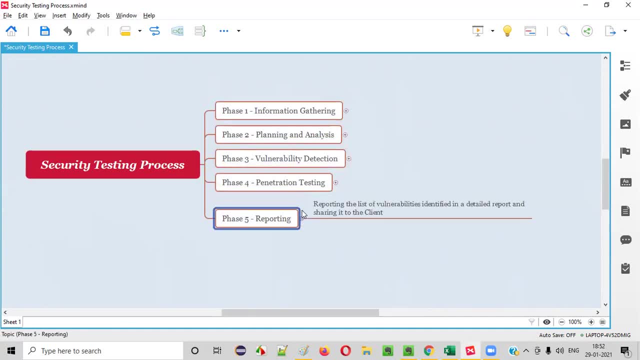 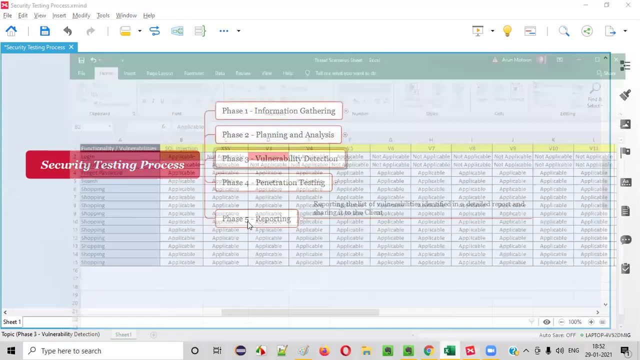 what are the different phases of this secure testing process? fine, so this report you can create in a better way if you have good knowledge about different type of vulnerabilities we have. okay, uh, till now i didn't explain about different vulnerability types, right, so i'm i'll be starting. 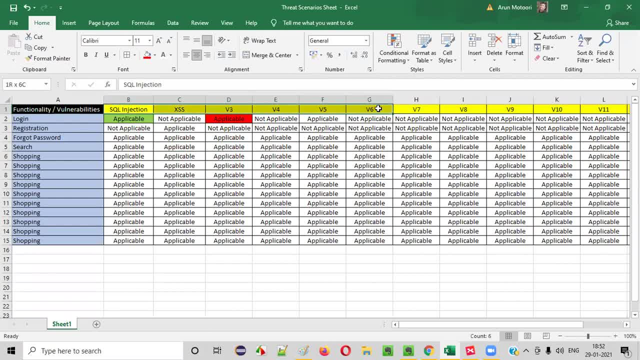 soon, guys, in next one or two sessions, we'll be going to the different type of vulnerabilities. okay, we'll start with the list of vulnerabilities and we'll go through each. we'll go through each and every vulnerability, like what is sql engine and, okay, how to perform it, how to detect it, all the stuff. okay, with lots and lots of examples. i'm 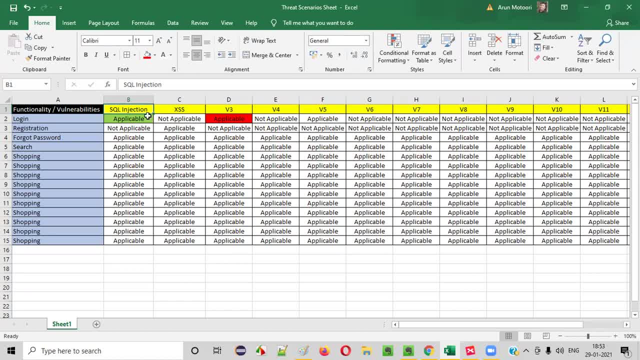 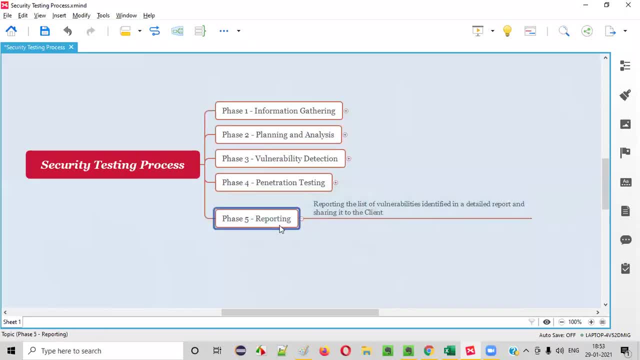 going to show you in the upcoming sessions, guys. so till now we didn't get a good knowledge about this, i didn't share any good knowledge about these vulnerability types. but, uh, once you get that good knowledge about the vulnerability types and their impacts and all those stuff, okay, then you can. 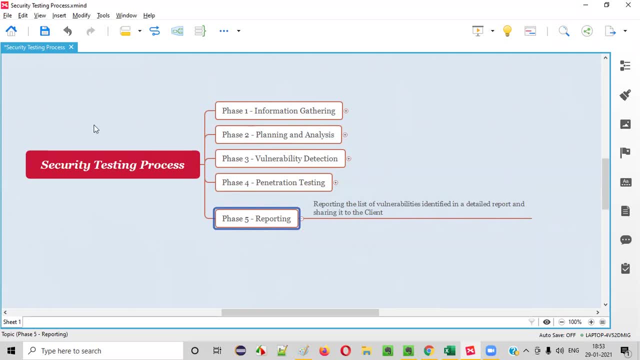 create very good reports. okay, then you can create a proper report, security kind of, uh, security type of reports you can create based on that knowledge that you will get after a few sessions. okay, so once, uh, okay, this is the last phase, guys, reporting is the last phase. okay, reporting is the. 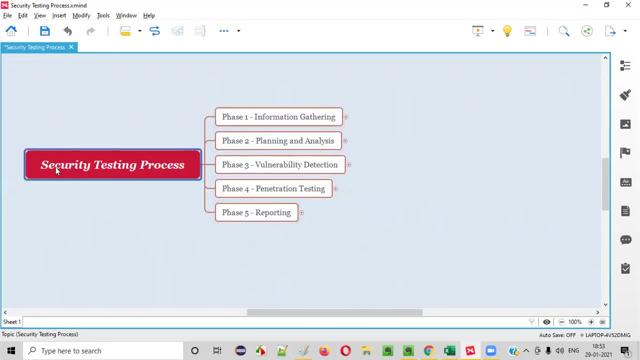 last phase. anyhow, all these phases, whatever i explained here in this security testing process that i'm going to show you practically in the upcoming sessions as part of a live project- okay, when the time comes, after we learn all the different type of vulnerabilities and how to detect.